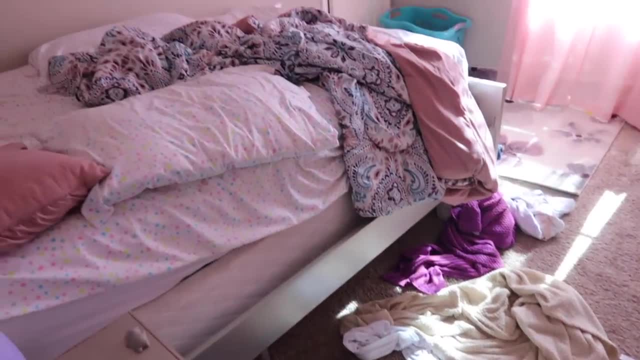 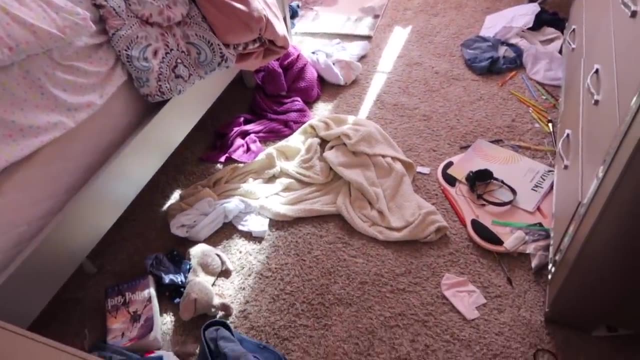 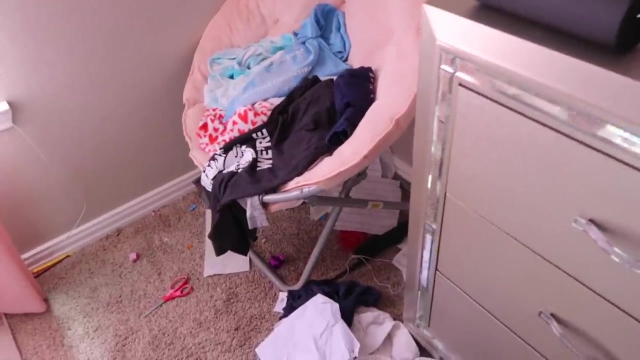 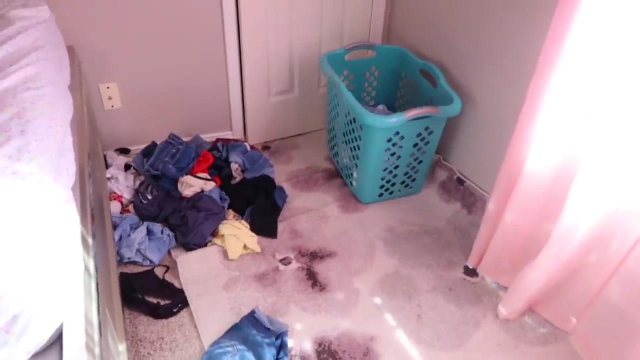 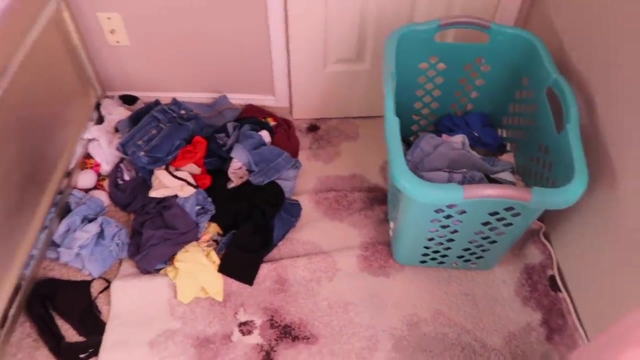 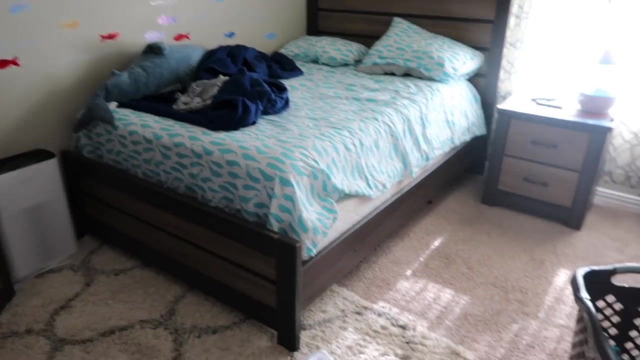 Hey guys, it's Karima, and welcome back to another cleaning motivation video. This time we are going to tackle the kids room, starting with my daughter's room first. You guys know it takes me the most time to clean and organize her things. Then I'll jump over to Kingston's room. It's a lot easier in. 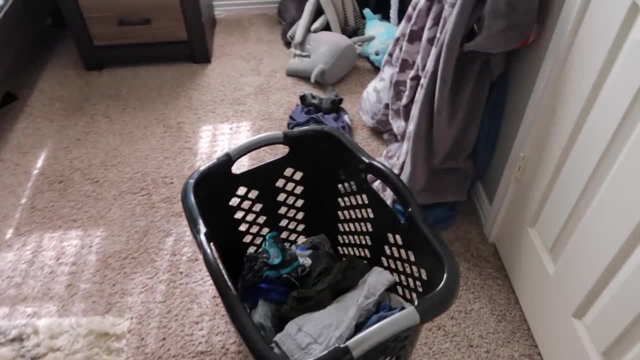 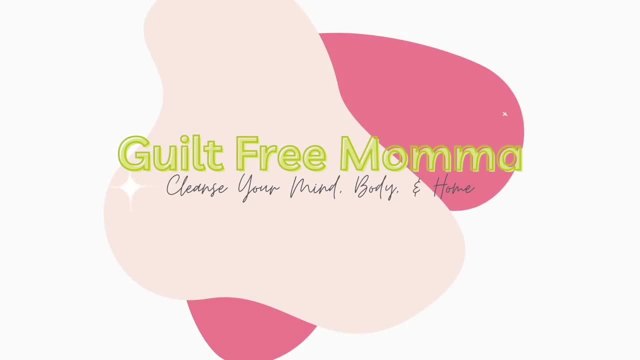 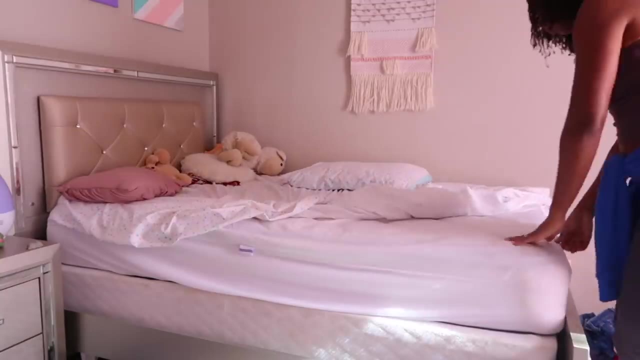 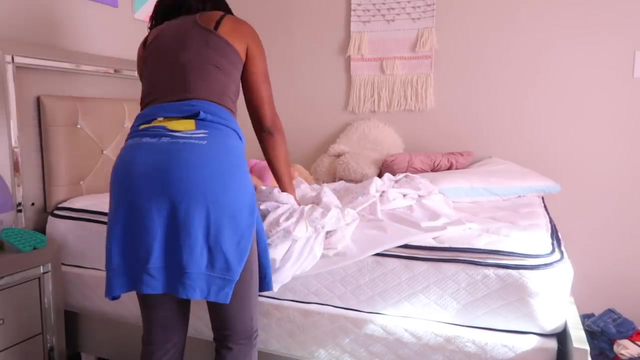 there, but we will be getting everything done in this video. So I'm going to start out by washing her sheets and getting that going so I can have it on her bed by nighttime, But in this video we are going to be cleaning, organizing and decluttering. I didn't go through her clothes. 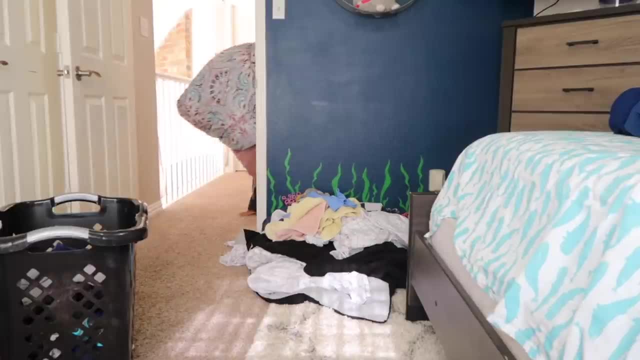 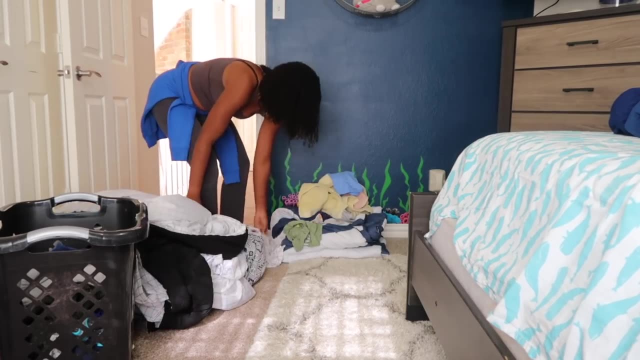 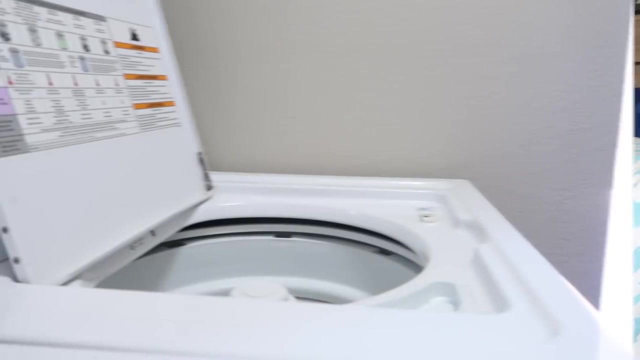 for school, so I'm going to do that. in this video, I'm also going to grab Kingston's sheets. I already changed his bed, so his dirty sheets are on the floor. I'm going to toss all of that in the wash. And before we get too far into the video, I just want to thank all my awesome subscribers who 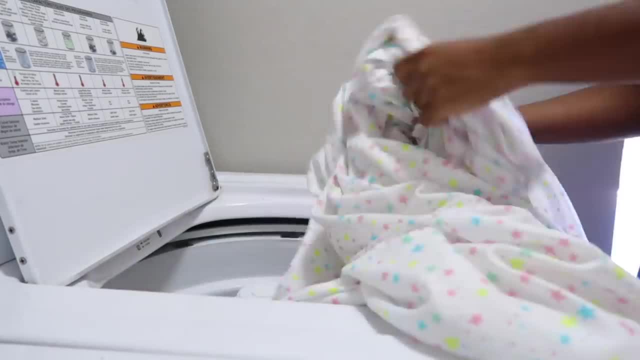 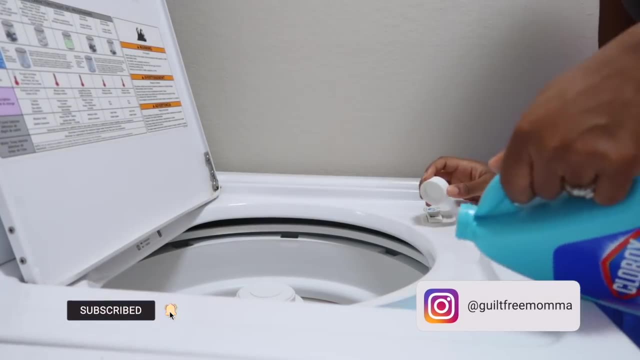 support me in every video. Thank you so much for the support and always watching, And if you're new here, please consider subscribing and commenting below. Of course. I really think you'll enjoy my channel if you're looking for realistic cleaning motivation from a working mom. 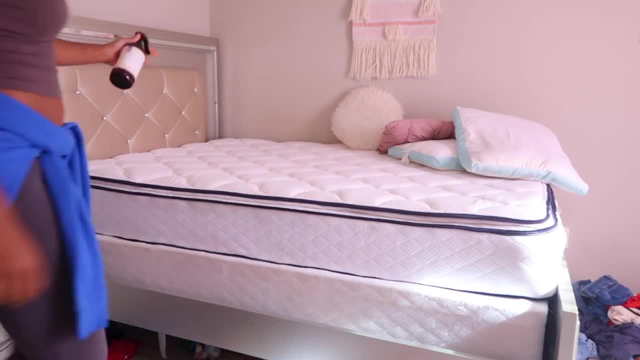 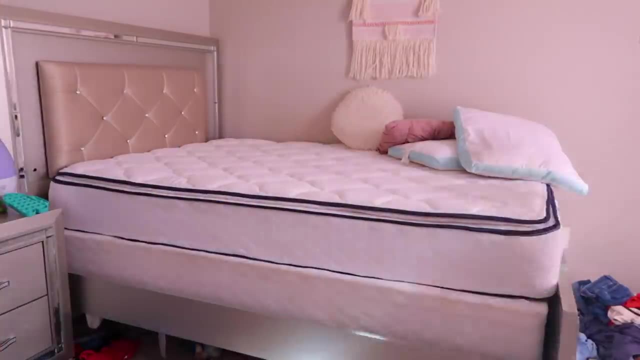 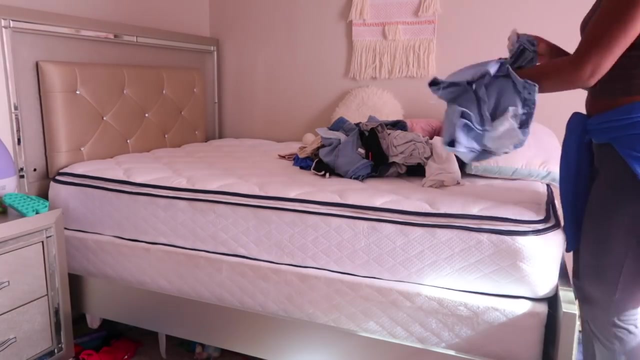 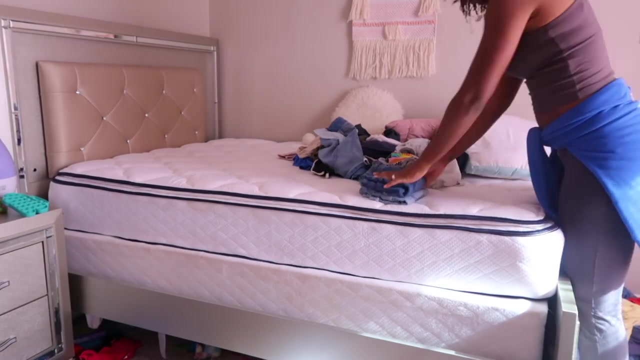 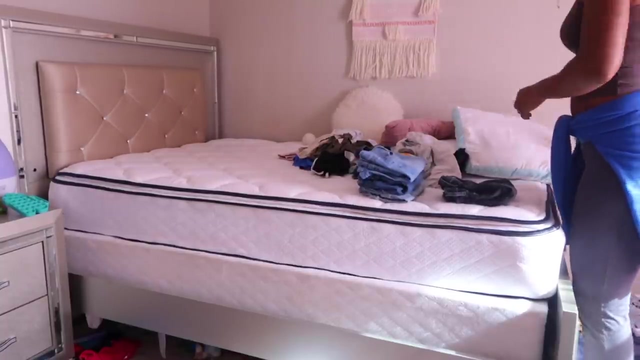 I had recently washed and folded her clothes and put it back in her basket to take upstairs and put away. That never happened. She just got dressed from the basket. I'm going to show you- and it's not her fault. You will see in this video why she couldn't properly put her clothes. 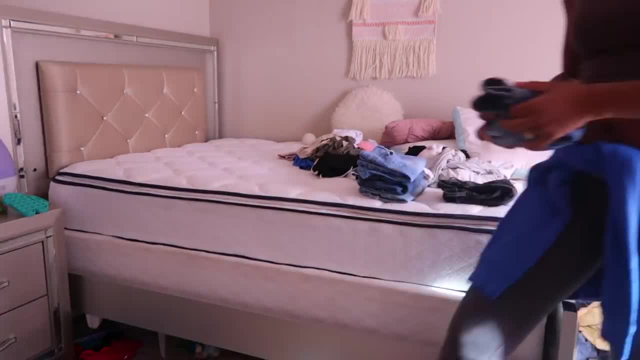 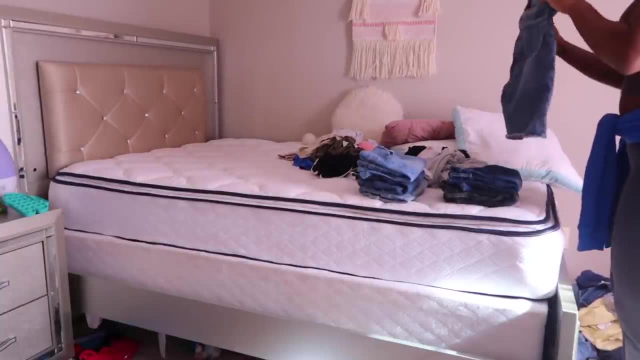 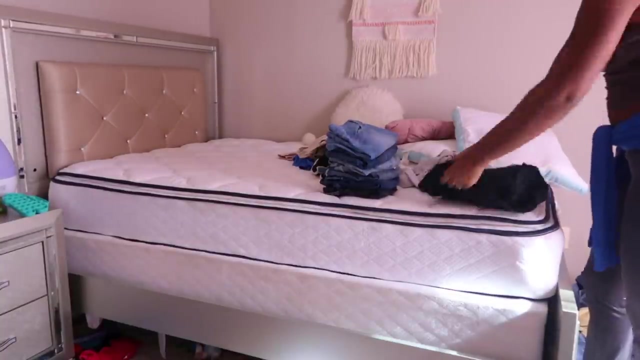 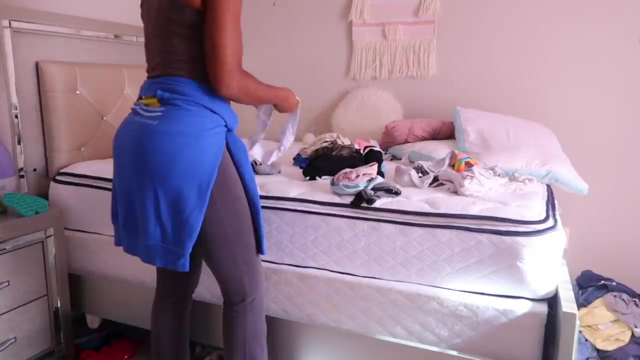 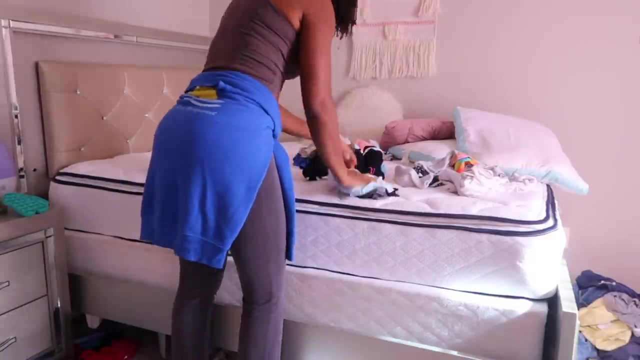 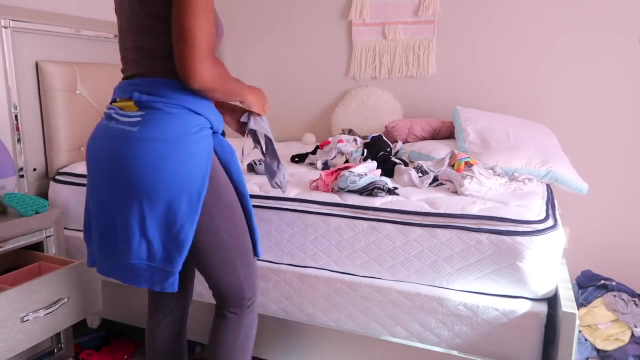 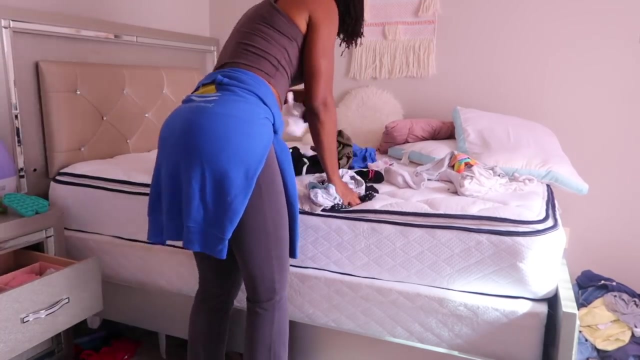 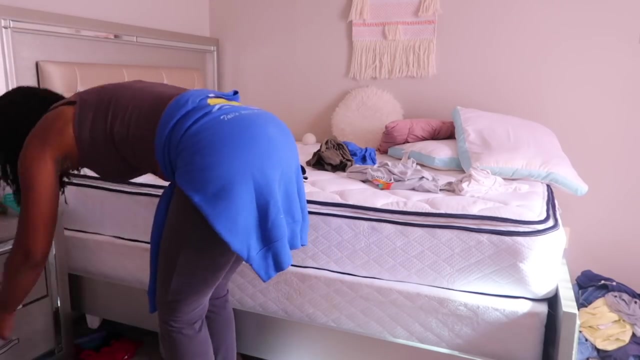 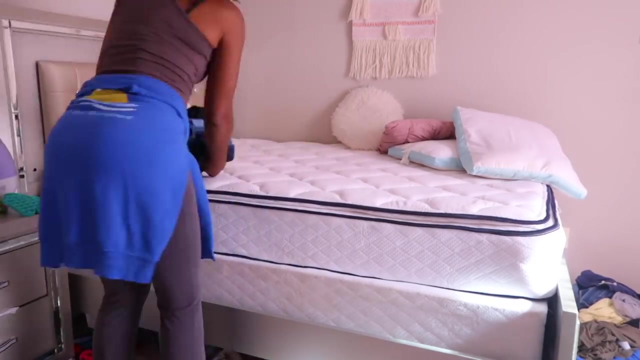 away. It's partially her fault, but it's partially my fault as well, So I'm just going to help her take care of that. I'll see you guys in the next one. Okay guys. so I came to put her clothes in her drawers, and this is what they look like. 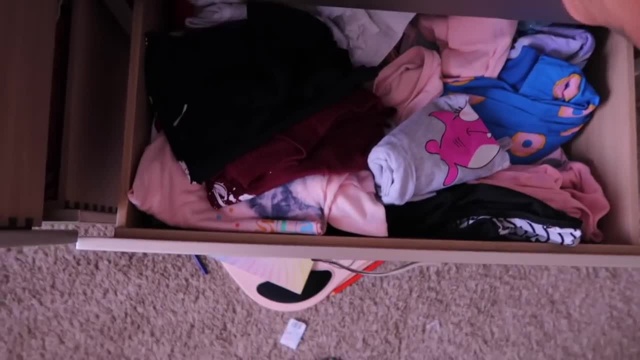 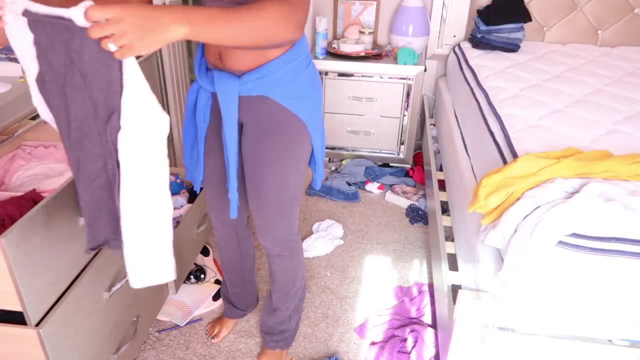 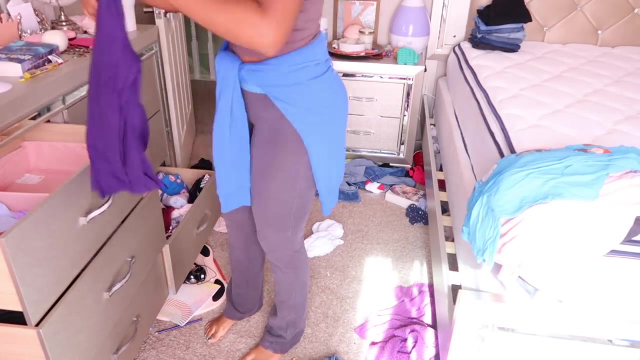 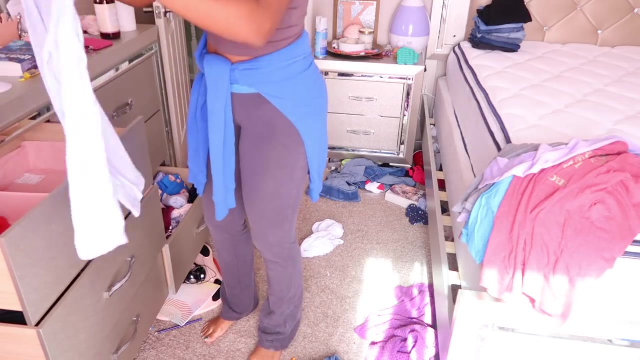 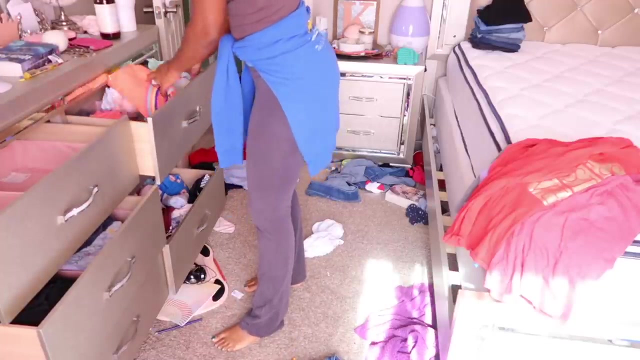 Okay, so of course, nothing that I put in is going to fit, so I am going to fix this first. So now that you've seen the inside of her dresser drawers, you can see why I said it was partially my fault that her clothes weren't put away, because I didn't go through her clothes for the summer. 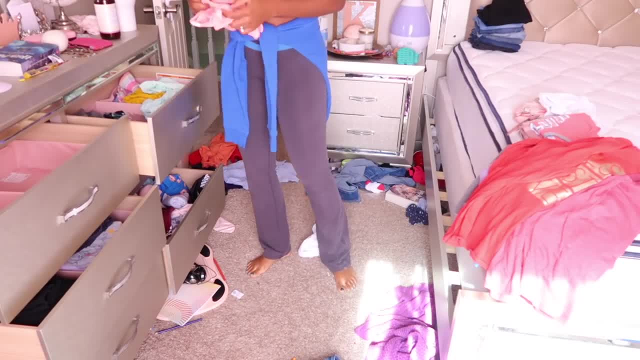 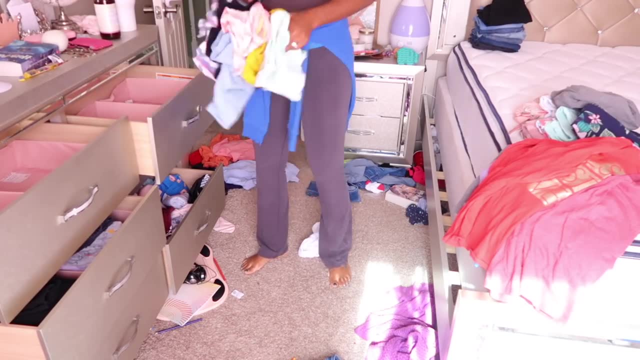 season, or or the back to school season, to be honest. So there were a lot of things in there that she just wasn't wearing, that was pretty much taken up by her. So I'm going to show you guys a space in her drawer. So right now I am just going through everything. I'm going to take out all the 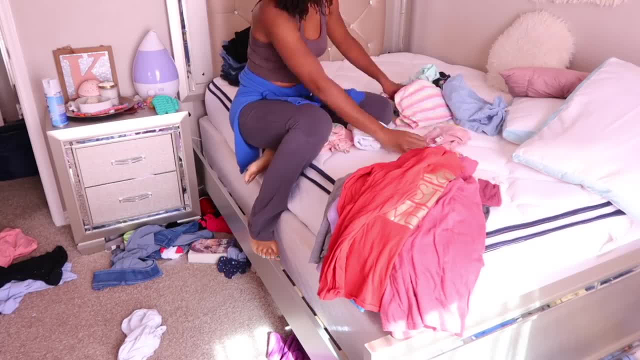 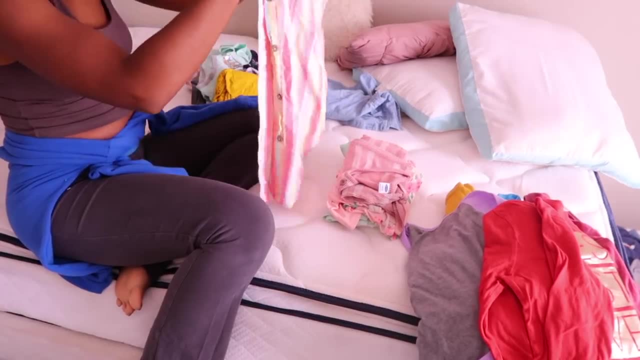 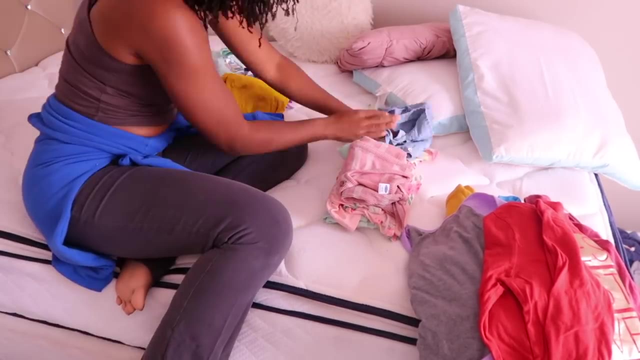 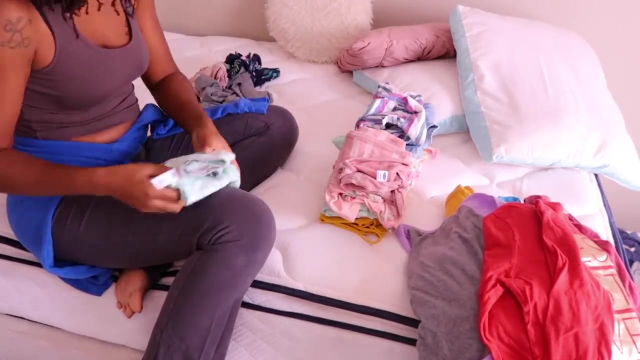 things that are either too small for her or I know she doesn't wear. I'm going to refold her clothes and we're going to have a nice conversation about making sure she puts it in folded nice and neatly, And so I'm just going to show you guys where the things that are supposed to be in there are. 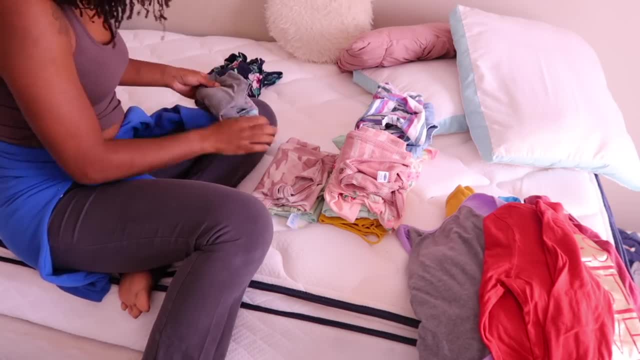 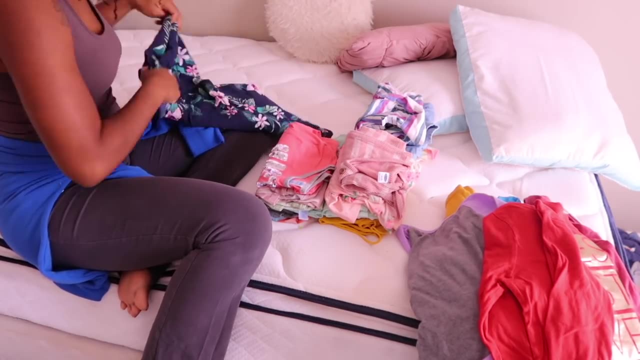 I'm going to go to the second drawer. So this is a drawer that has some stuff that's been in there. But I'm going to go to my new drawer and I'm going to walk you through the things that I took out. So I'm going to have a little look at the new drawer. So there's a shed. It's a little bit smaller. 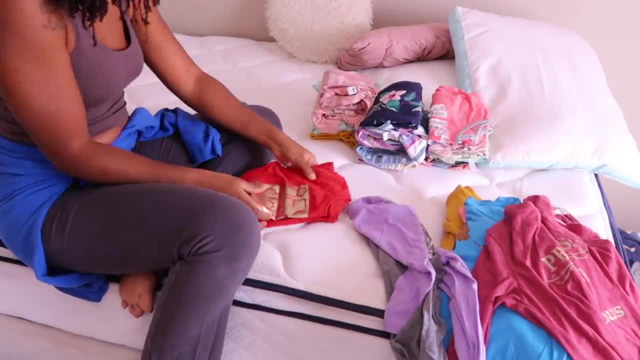 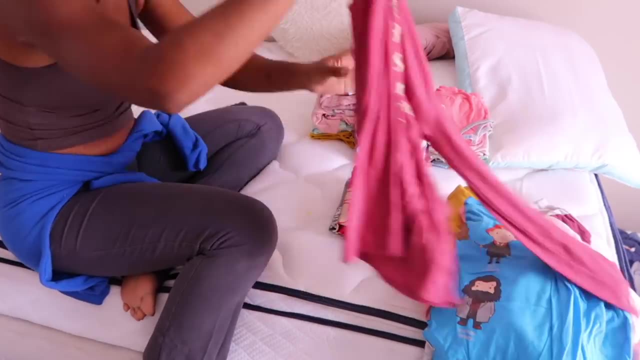 than the previous drawer, And then there's a little empty corner that I just put in there to help with the storage, And I'm going to take a look at the inside of her clothes and there's a little thing that is almost too big for her. So this is what she's doing And we're going to wrap a dresser. 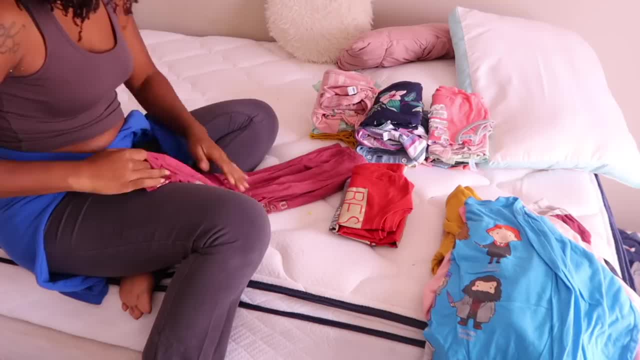 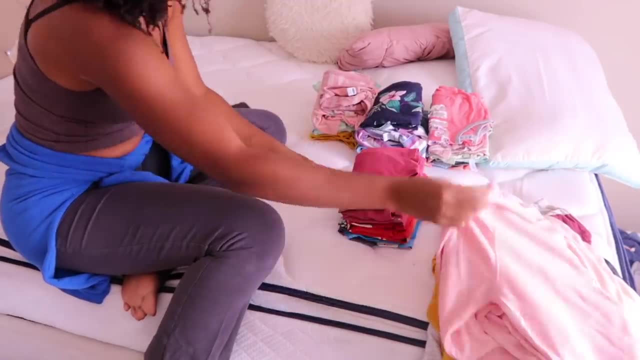 So right now, she's just going to go out and I'm going to go through the drawers. So, as you can see, it's all. so, guys, I'm finally going to commit to a posting schedule and I want to share it with you guys in this video. I also want to get your help with the perfect time. 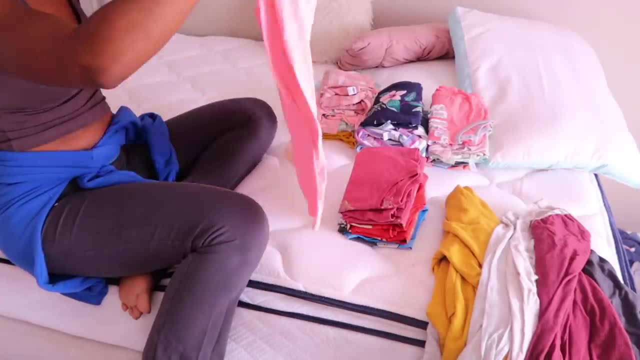 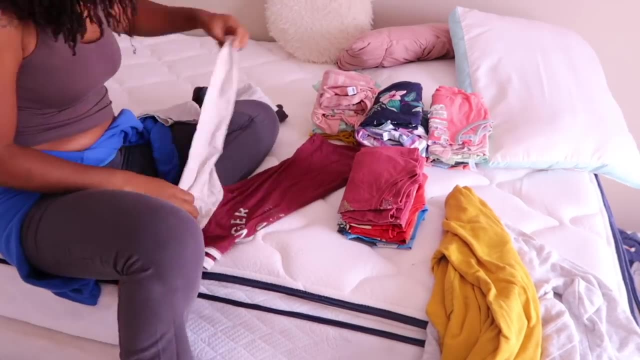 to post. so I think I am going to start posting on Thursdays and Sundays. I like the idea of Sundays because it's kind of the day that most people use to reset for the week anyway, and now that I don't work on Sundays anymore, I don't work. 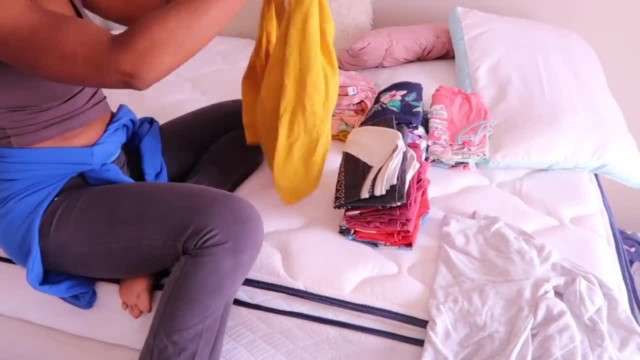 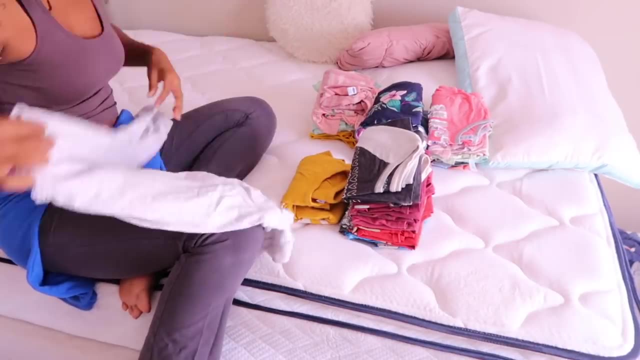 weekends anymore. for the most part, I like to use my Sundays to reset as well. so if I start posting on Sundays, what's a good time? I kind of have my time slot that I like for posting during the week. but do you guys like to watch your? 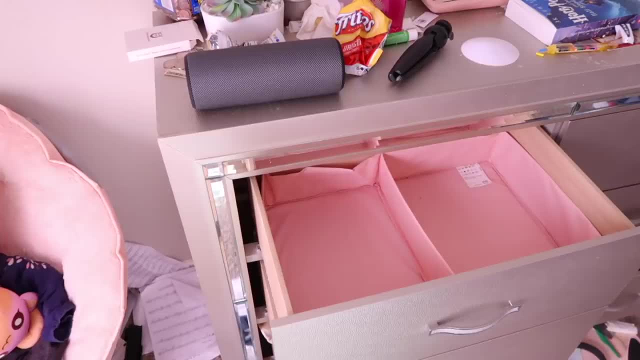 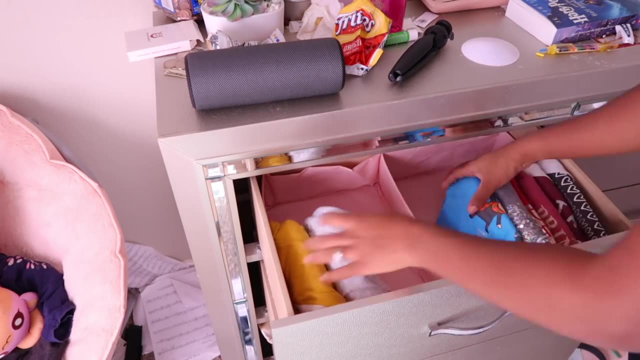 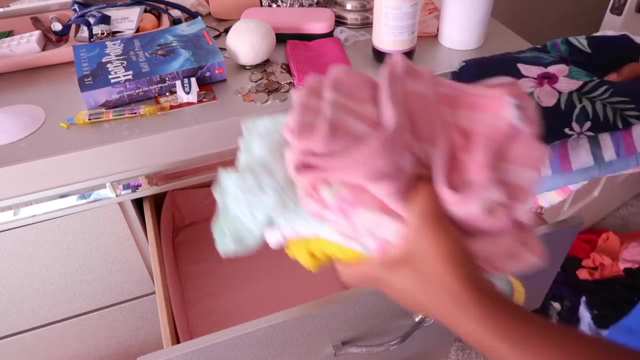 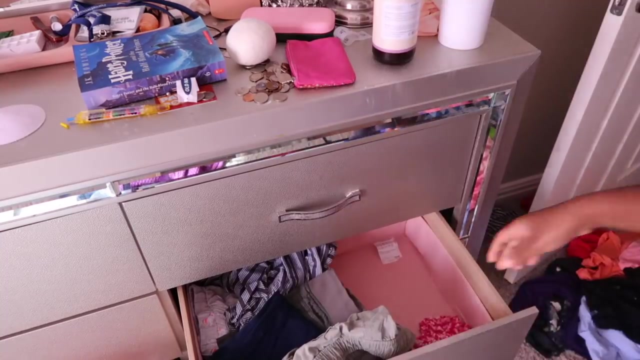 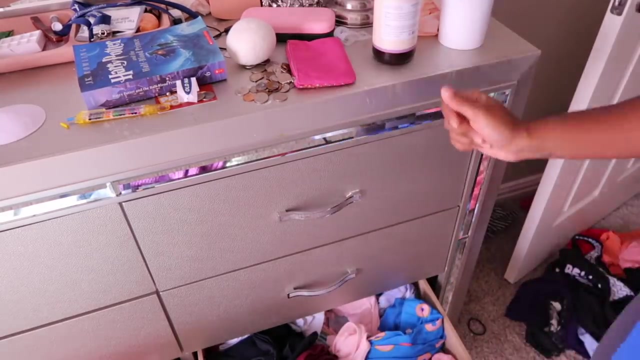 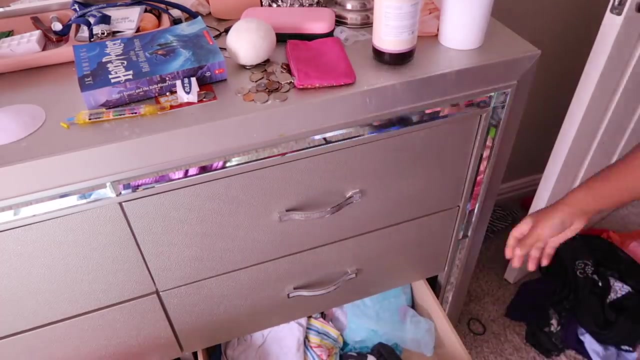 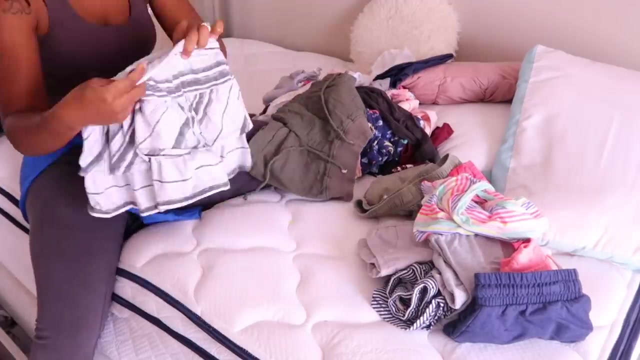 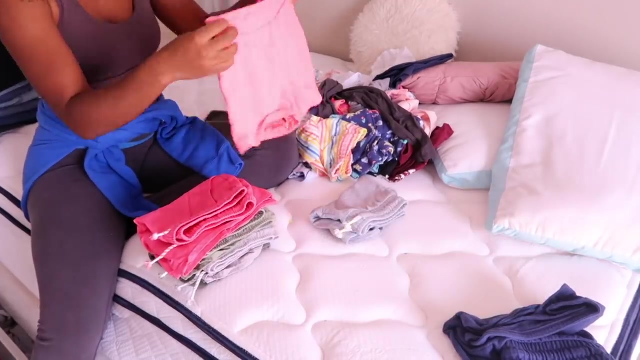 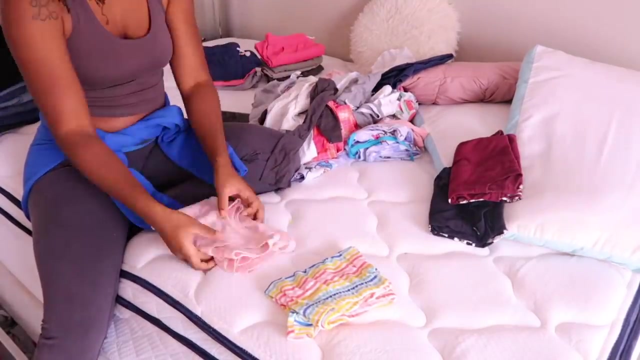 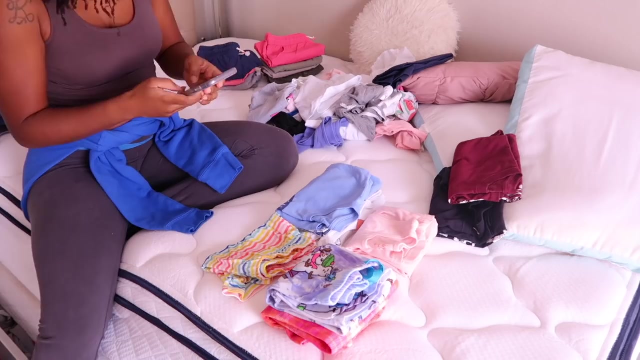 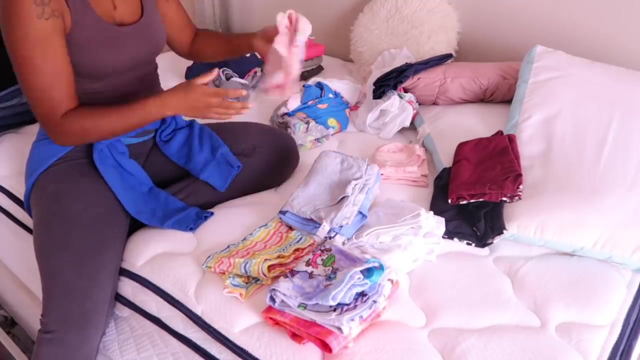 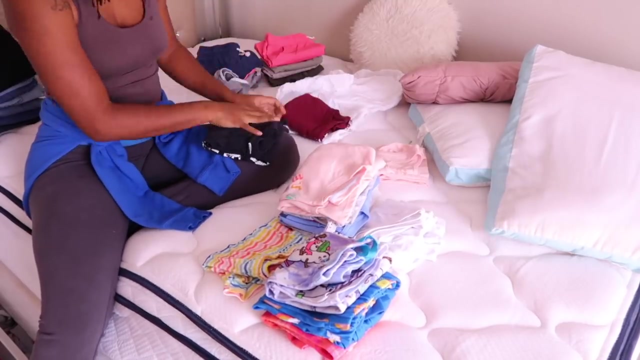 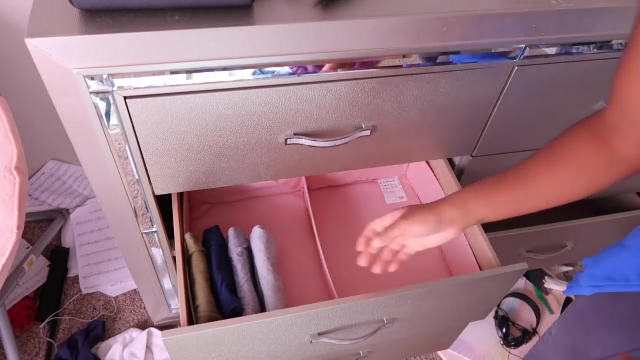 videos earlier in the morning, kind of in the afternoon, or do you prefer to watch it in the evening? let me know you, you, you, you, you you. so now that i got rid of all the clothes that's too small for her, or she just doesn't wear she. 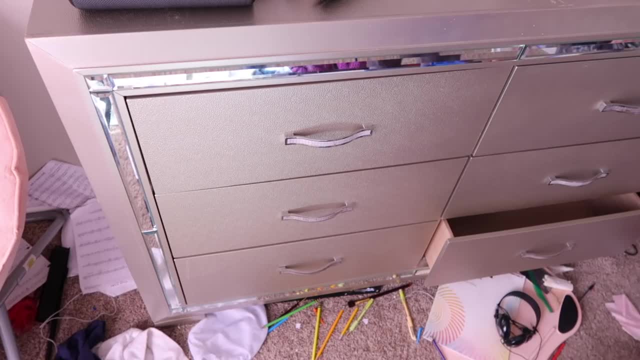 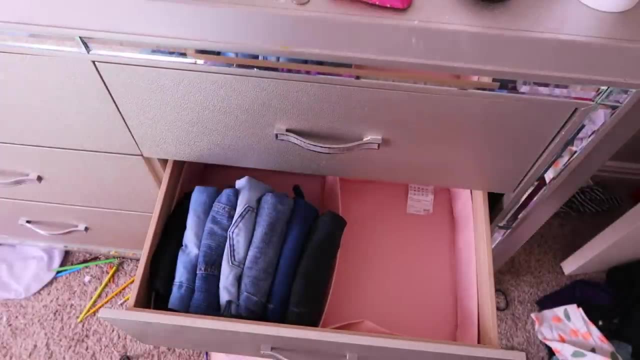 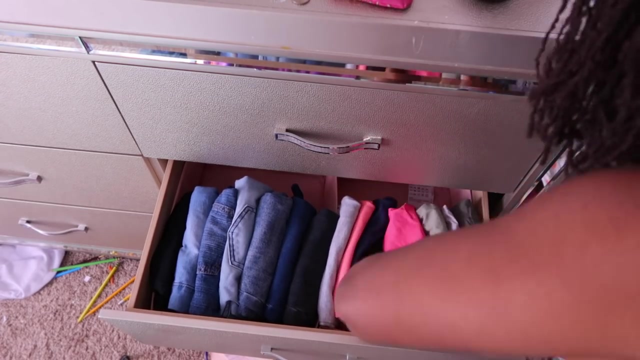 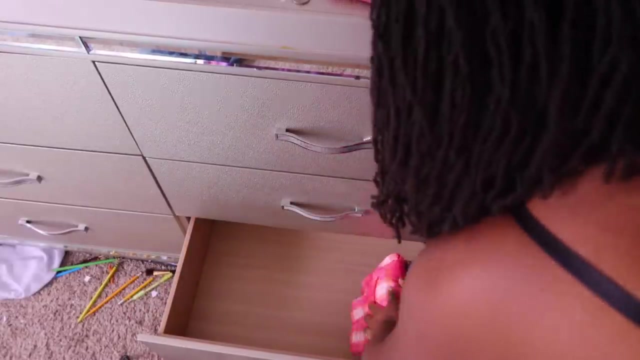 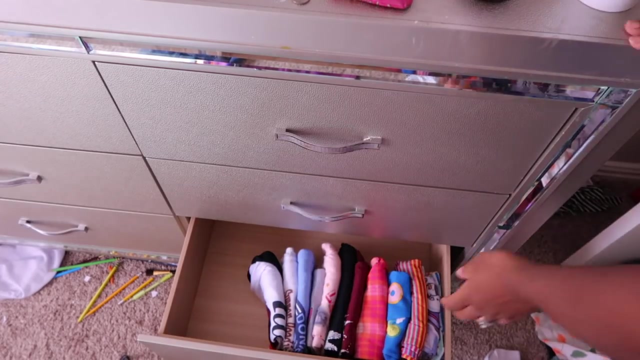 has tons of space in all of her drawers. all of them are pretty much half empty, excluding the clothes that may be in her dirty clothes hamper, so she has room to grow. she has plenty of clothes, though, so she's not getting anything new. so this is everything i cleaned out of her drawers that i know she 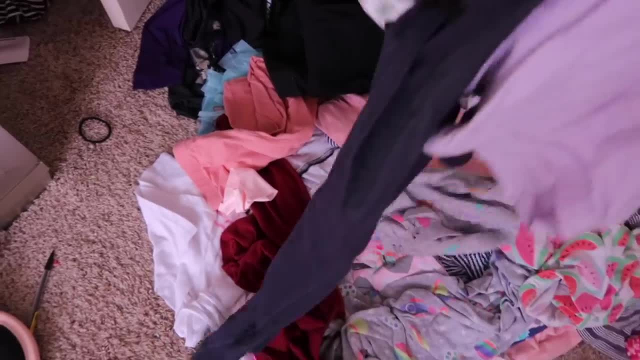 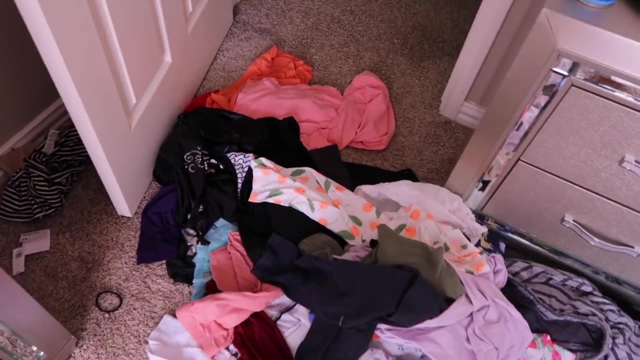 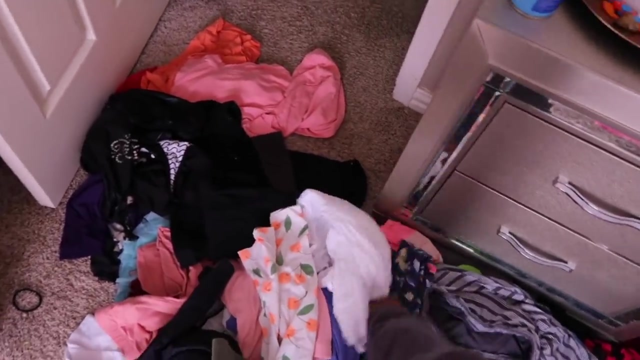 either cannot fit or will not wear. i didn't do that this season, like this school season, so it was about time because, as you saw, her drawers were like overstuffed in a mess, and partly it was because she had a bunch of things in there that really didn't need. 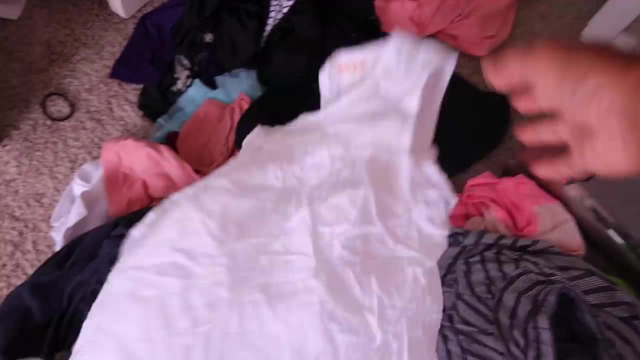 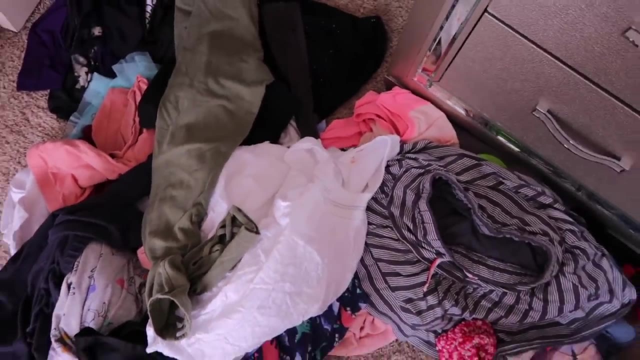 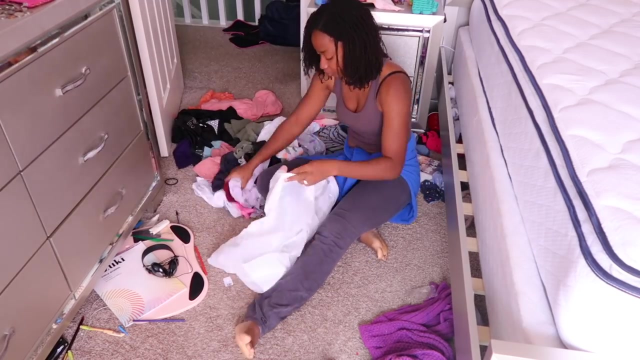 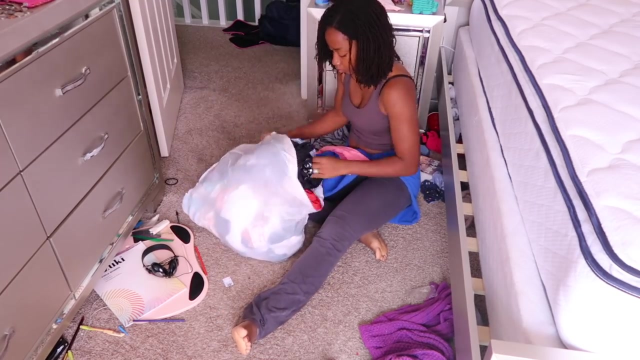 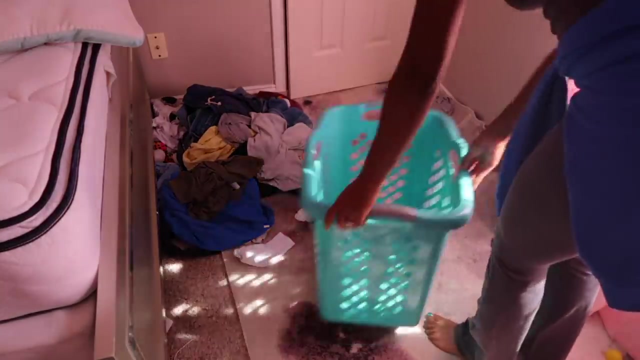 to be in there. i think she wore this top once. i love this top, but it's too small for her now. so these things, i will donate the good stuff and get rid of the not so good stuff. so, basically, because her clean clothes were still in her hamper, she just put all her dirty clothes. 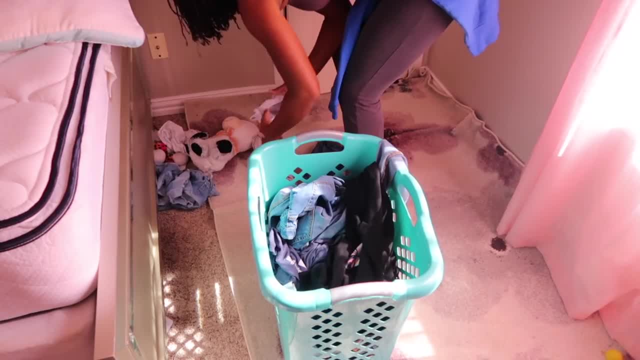 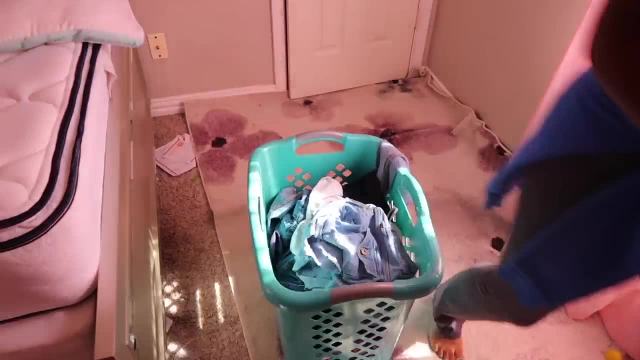 right there on the floor. i didn't stress about it because what else was she going to do? and before someone decides to choose violence in the comments, before i do spray out my kids hamper clothes and hampers with lysol, before i fold and put their clean clothes in it. we have but so many laundry. 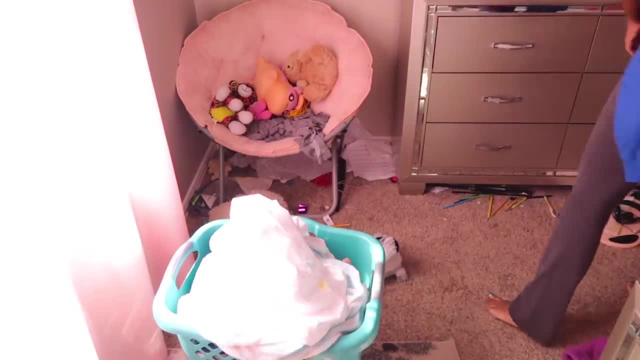 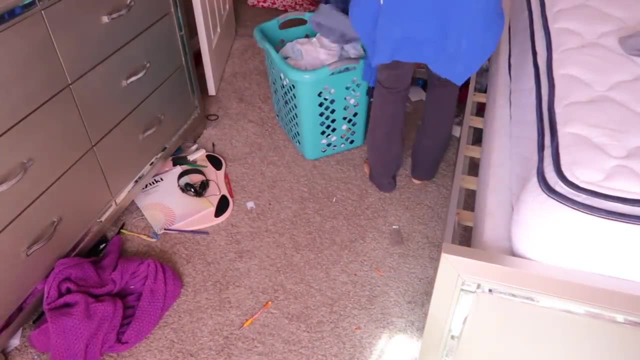 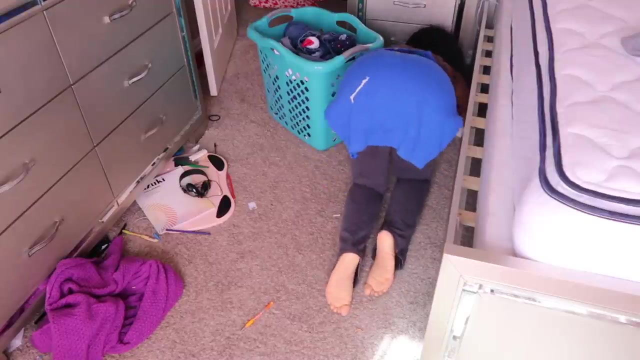 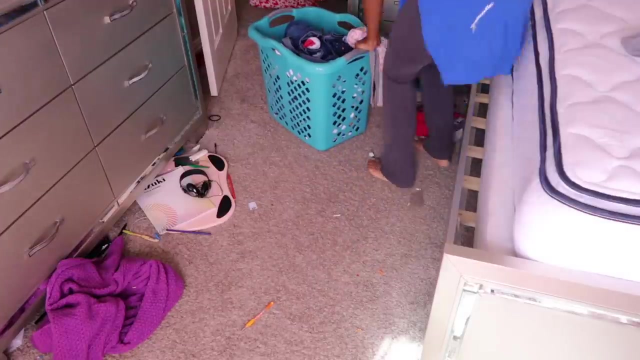 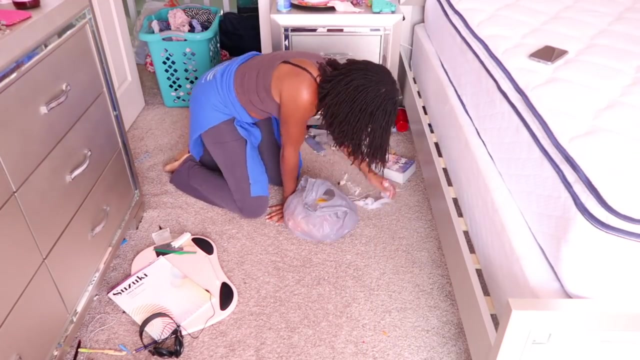 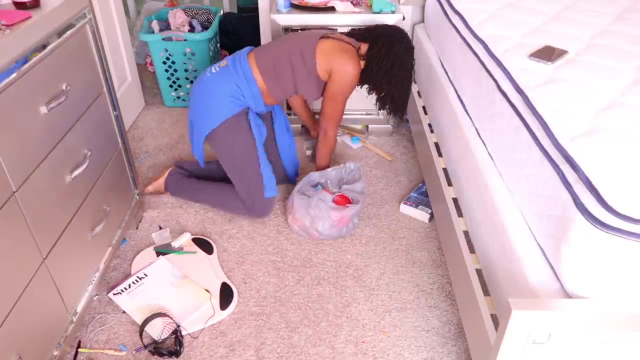 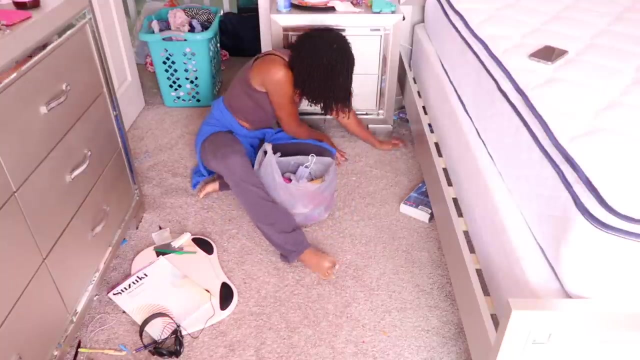 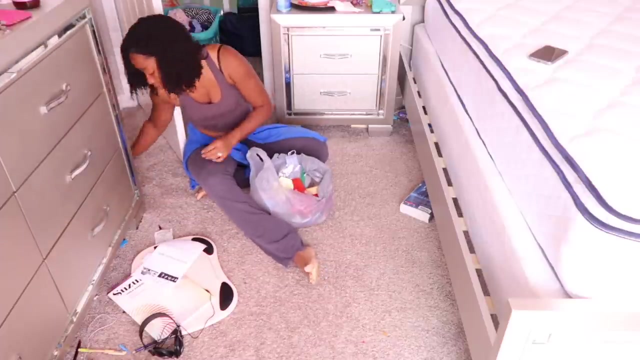 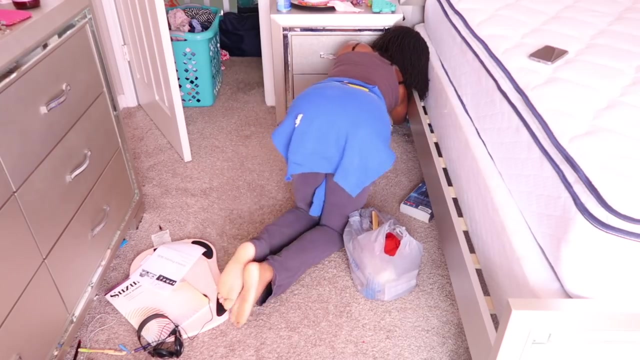 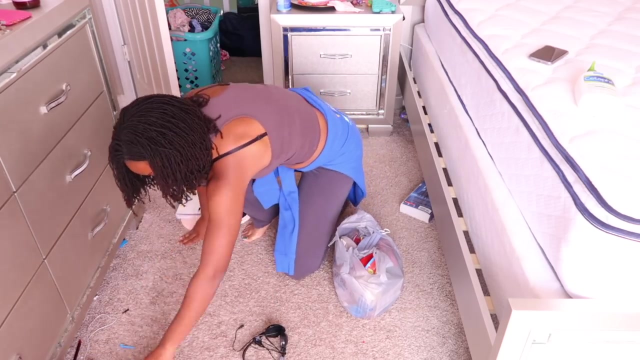 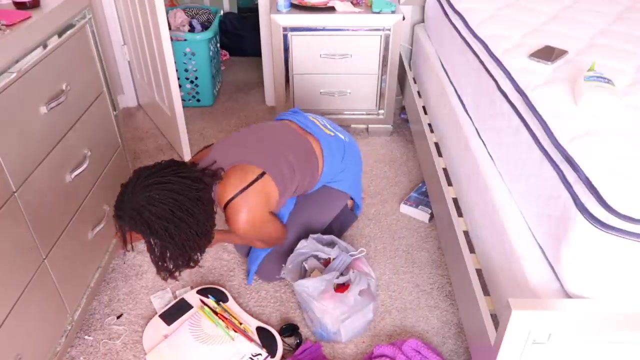 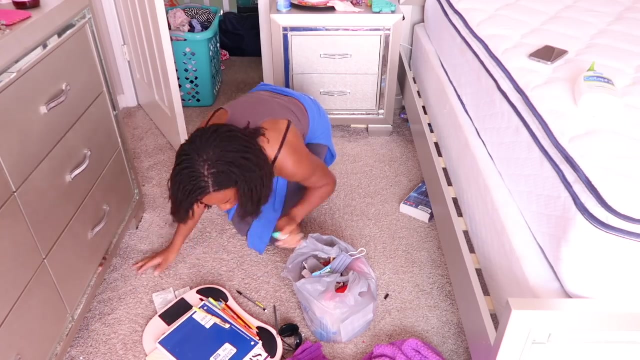 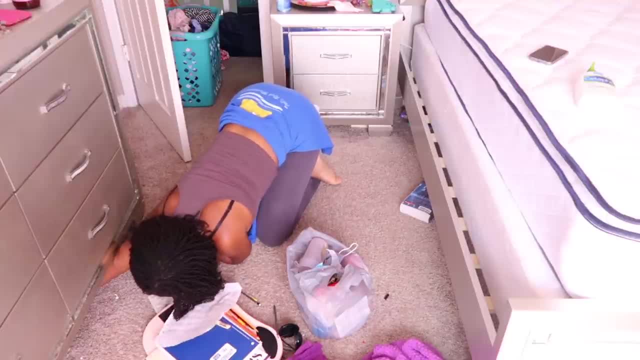 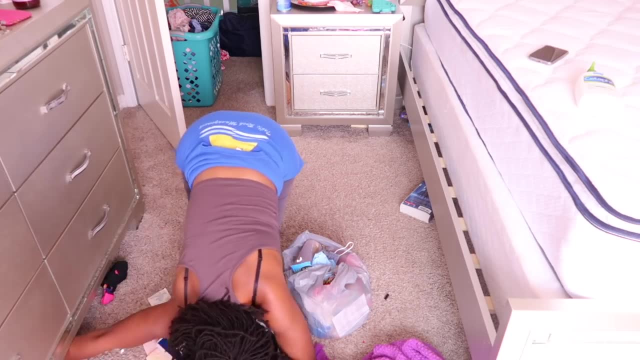 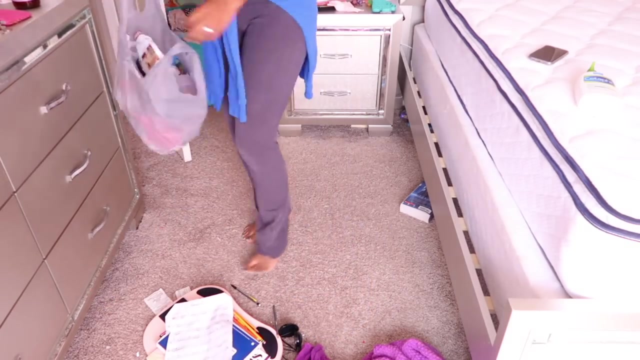 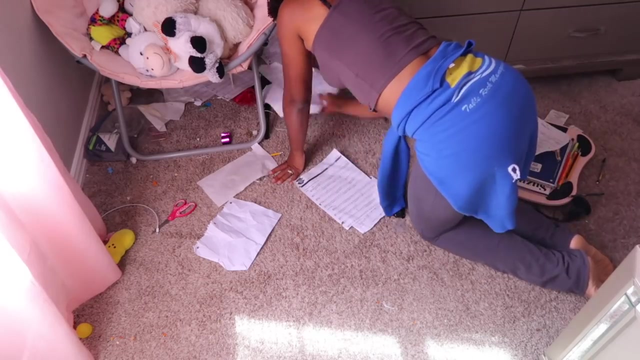 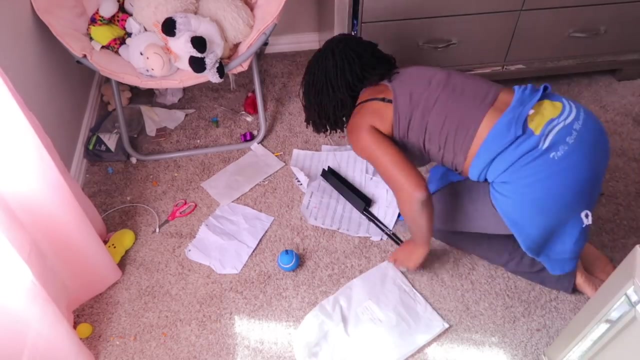 and if you're new here and you're wondering if i make my daughter clean her own room- of course i do. she's 11 years old. i do make her clean her room. i don't necessarily make her do it on camera though. well, i don't make her do it on camera because this is not her channel. and if it's not, 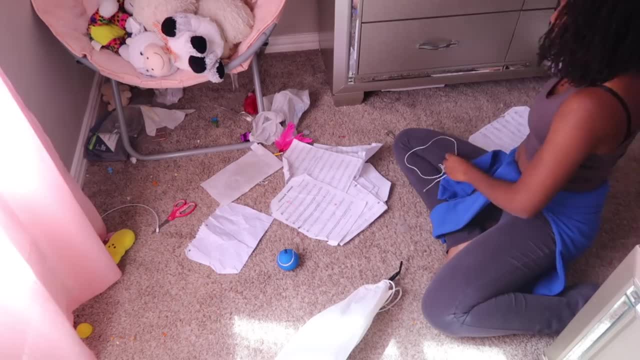 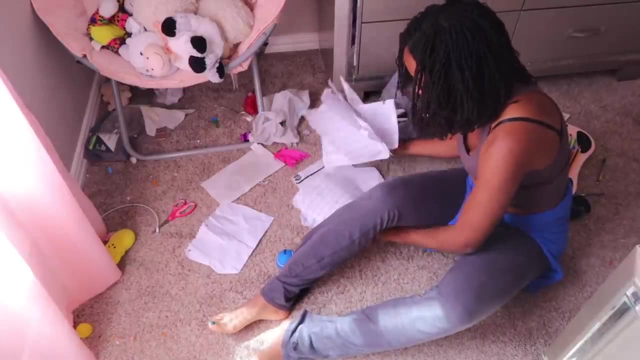 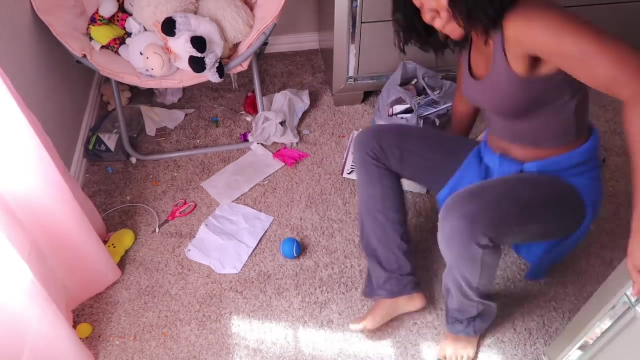 something she wants to do. sometimes we'll clean together on camera, but if she doesn't want to do that, i'm not going to make her do that. and also, she's a very busy kid. she's a great kid and she's messy by nature. she got it honestly. if you ever watch me clean my own room, you know that i am a 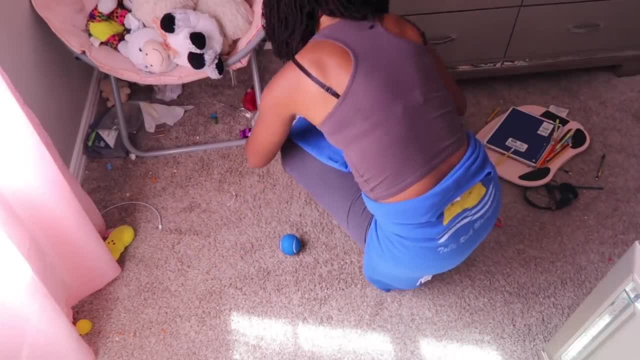 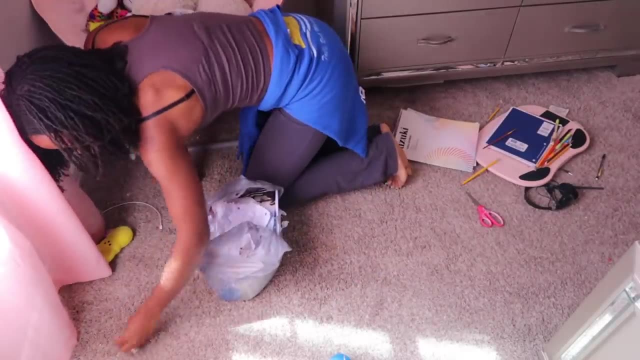 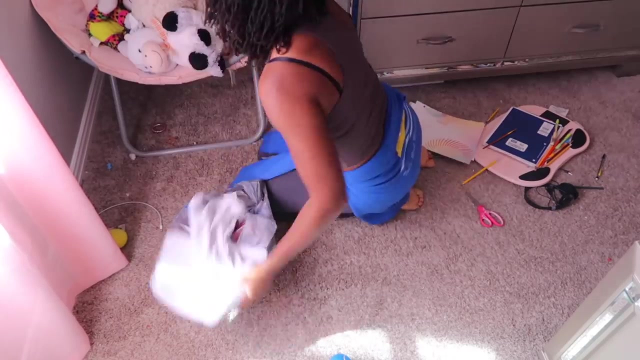 naturally messy person, so so is she, so it's. but so hard i can really be on her. she does make me work extra hard because she keeps a bunch of little things on the floor, so we do discuss those things, but at the end of the day i can't really go crazy on her because hey, then i'd be a pot calling the. 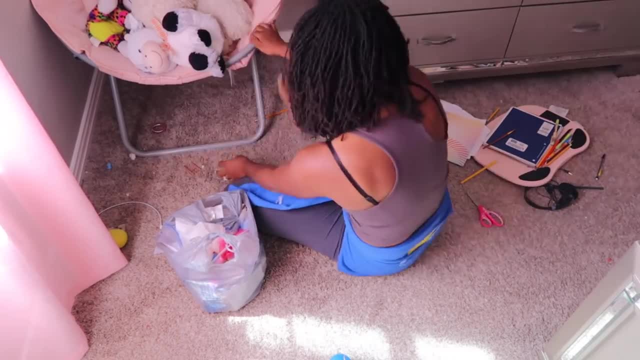 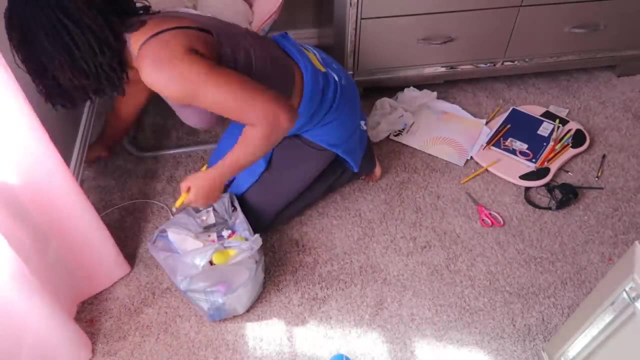 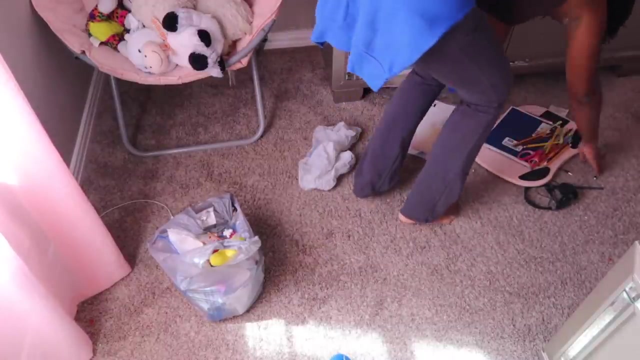 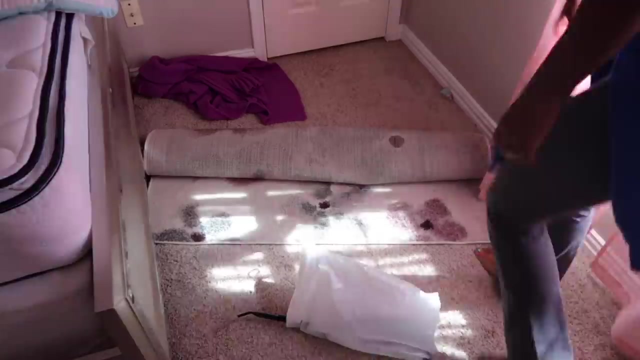 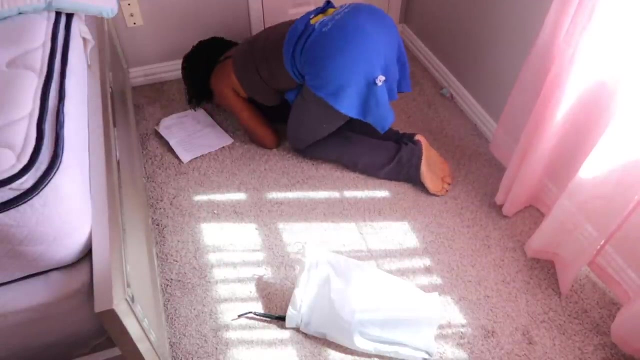 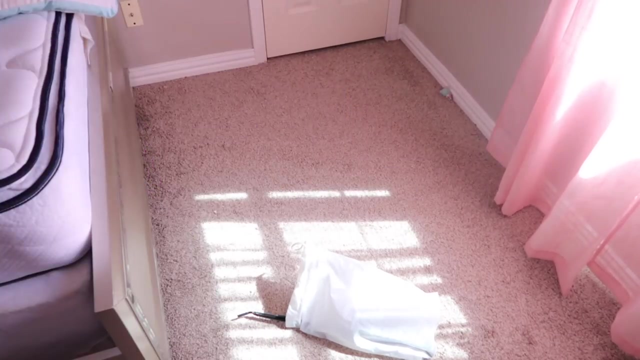 kettle black, so i decided to get rid of chloe's area rug. the edges were curling up so bad it was driving me crazy. and plus it would like move under her closet door and instead of moving it out, she would just close the closet door on it and it was jamming because of the hooks that were on top. it's. 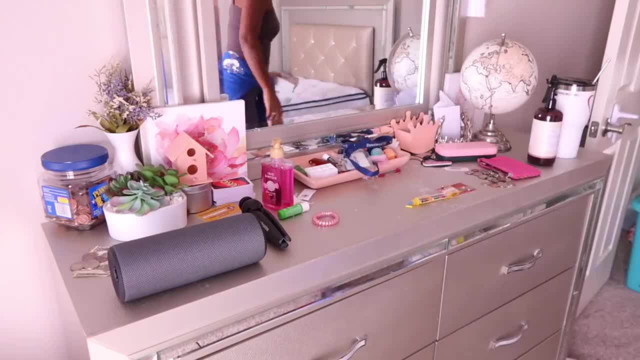 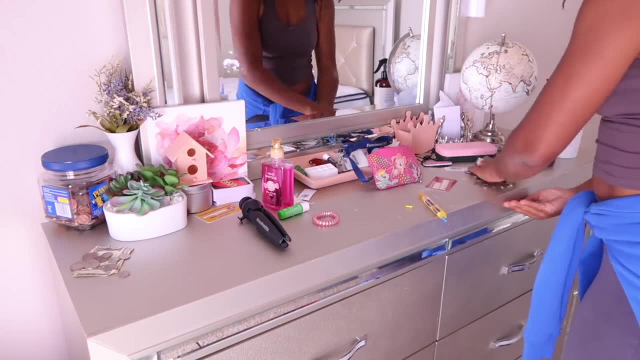 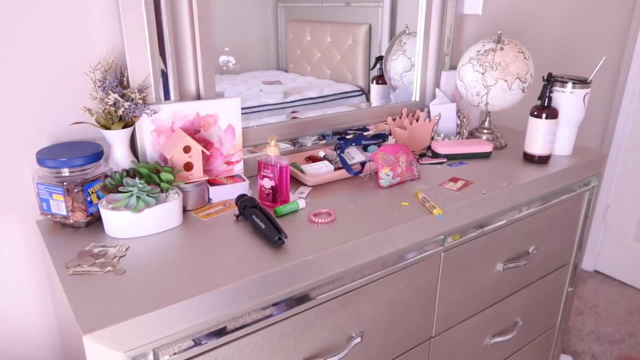 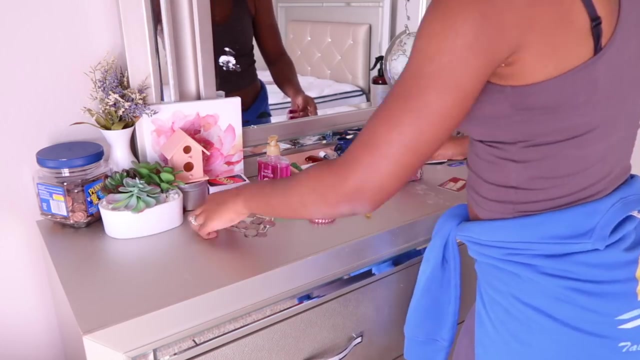 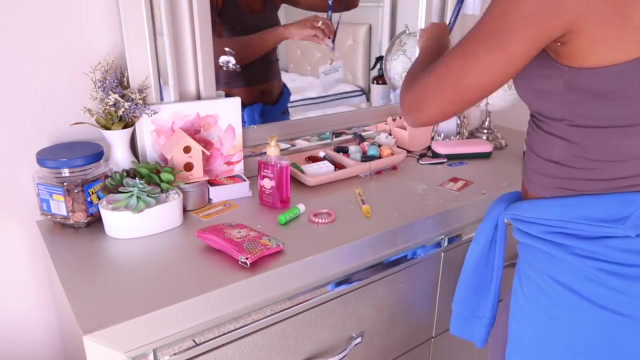 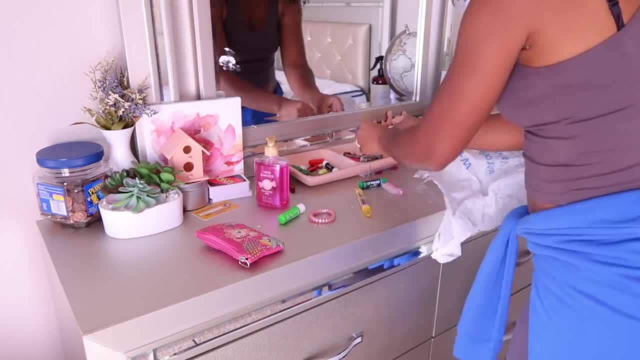 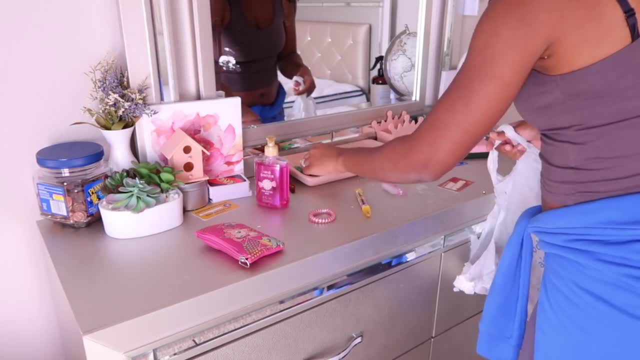 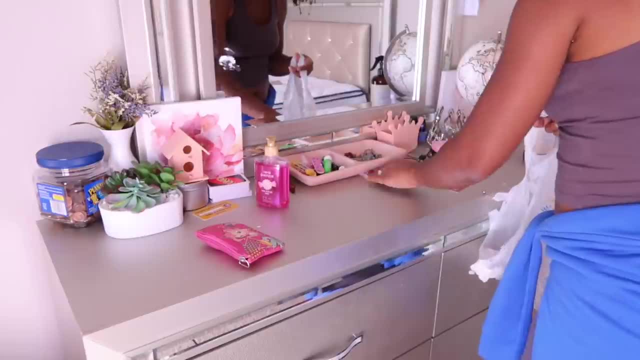 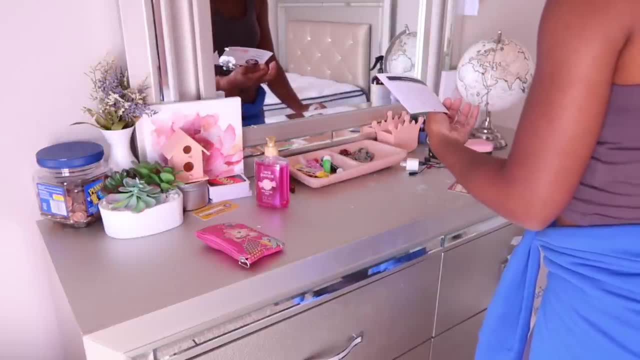 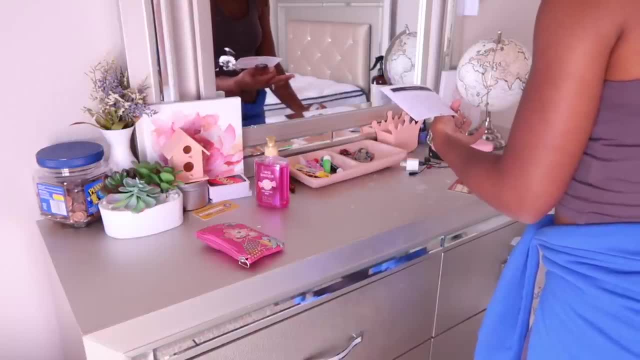 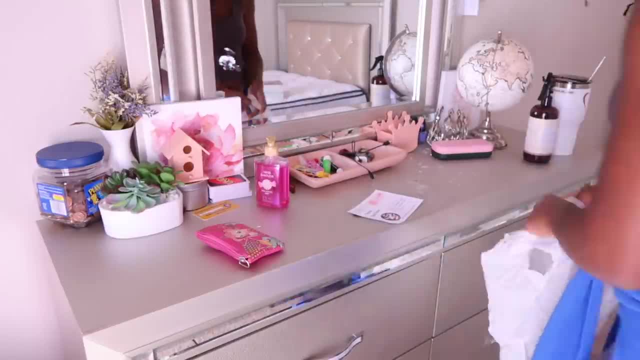 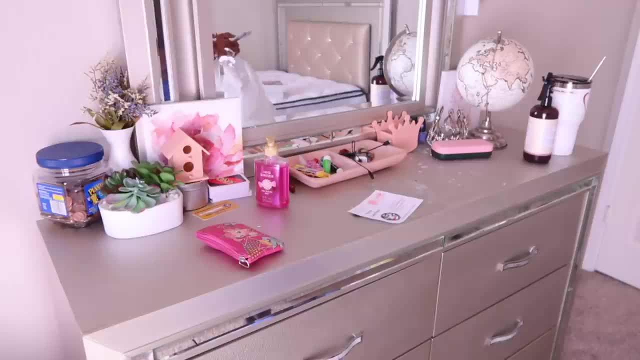 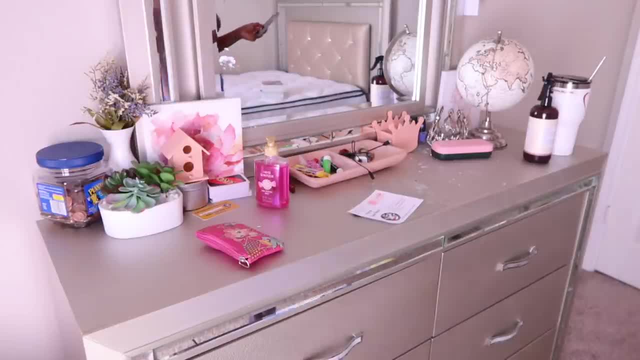 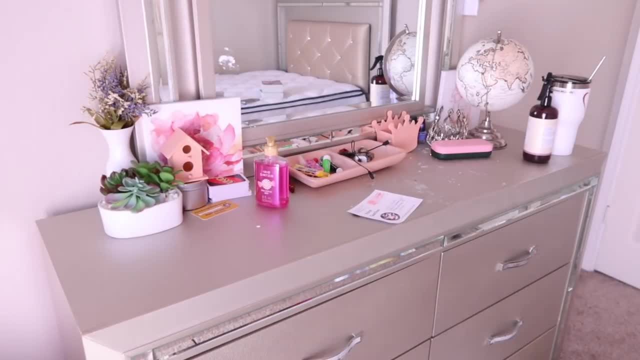 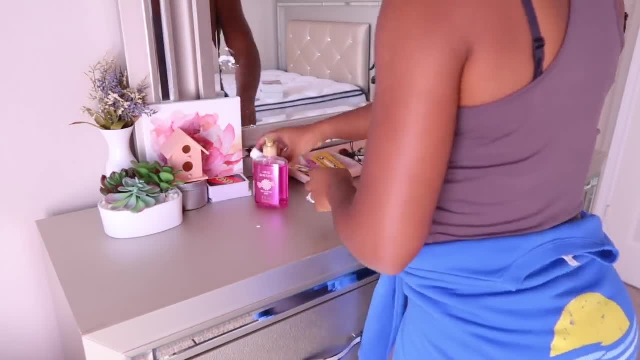 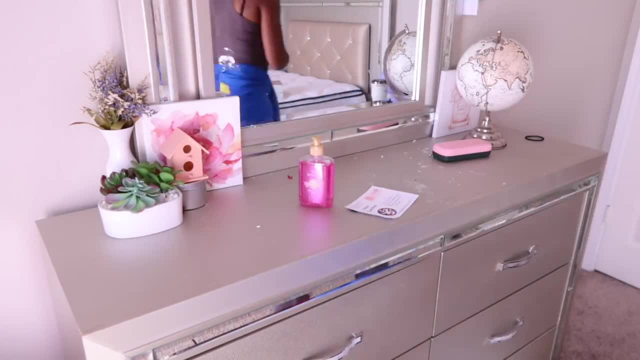 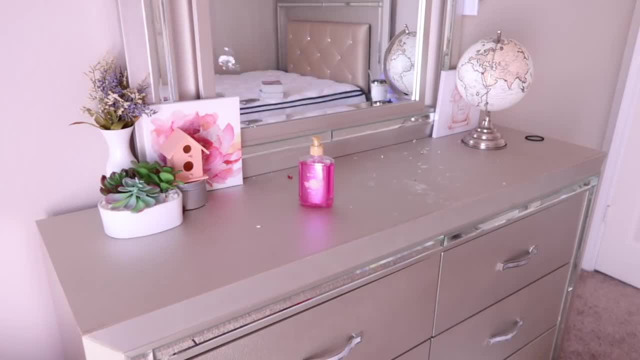 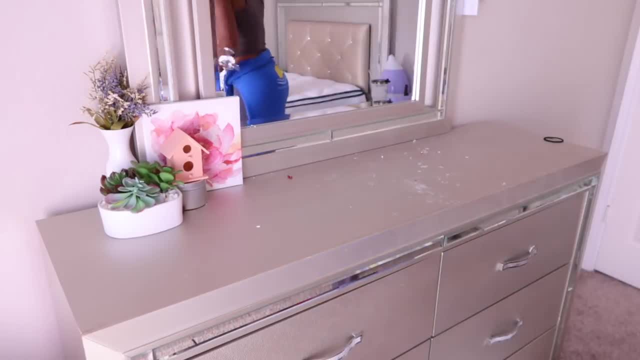 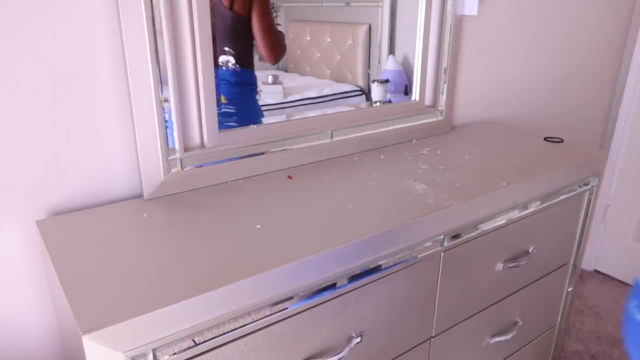 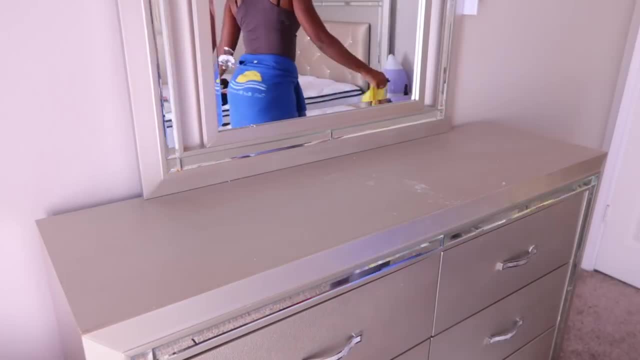 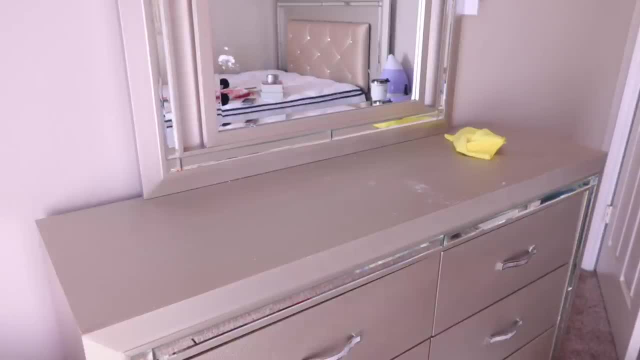 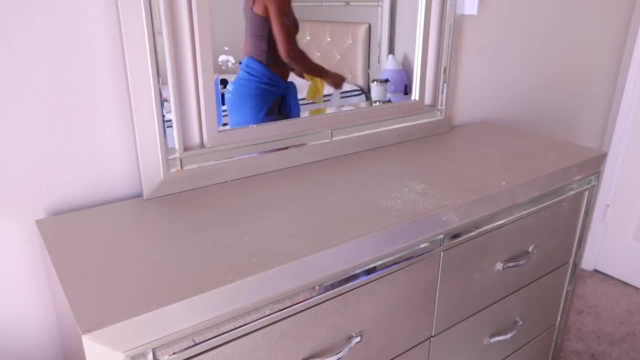 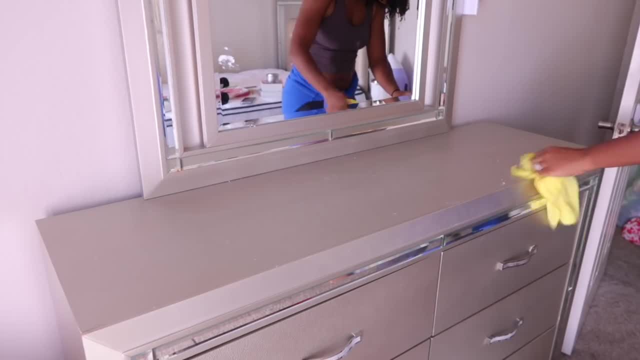 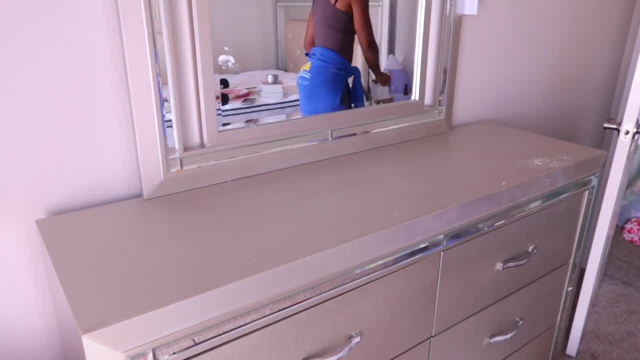 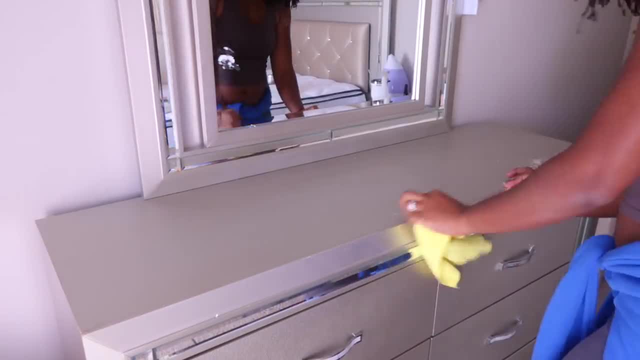 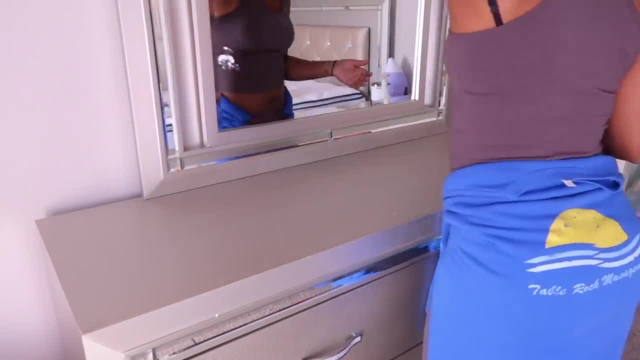 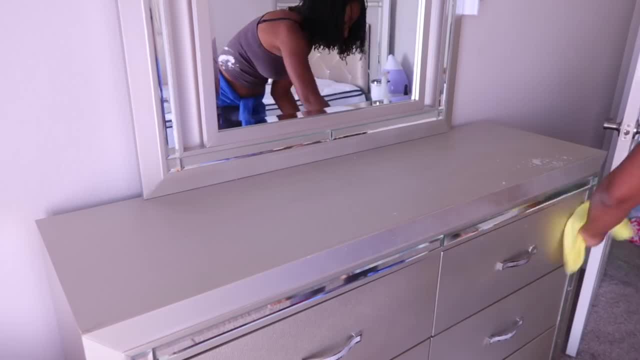 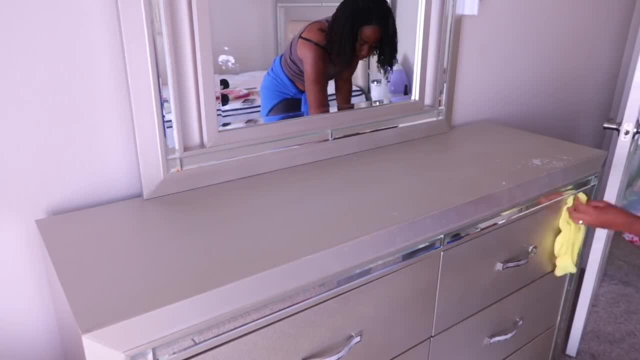 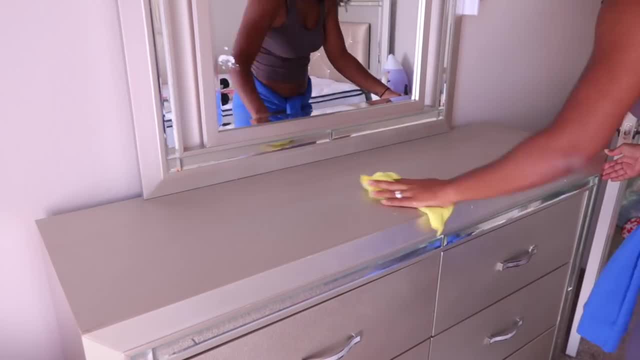 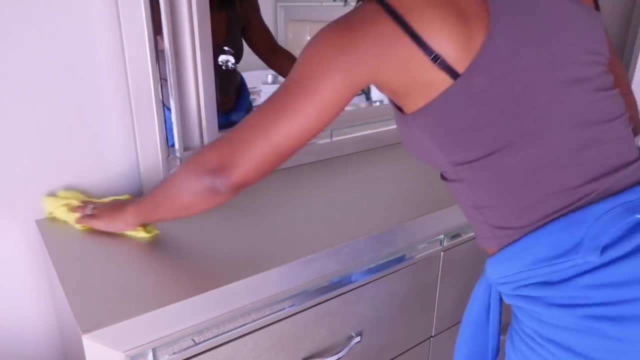 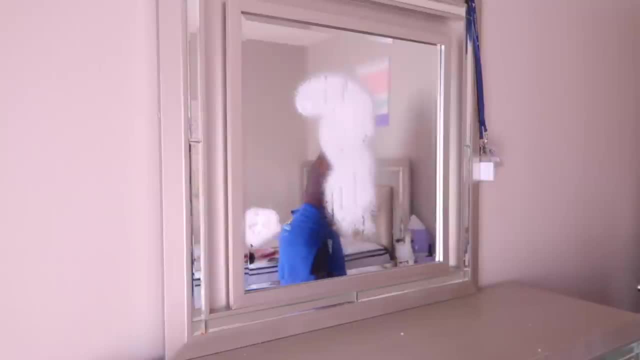 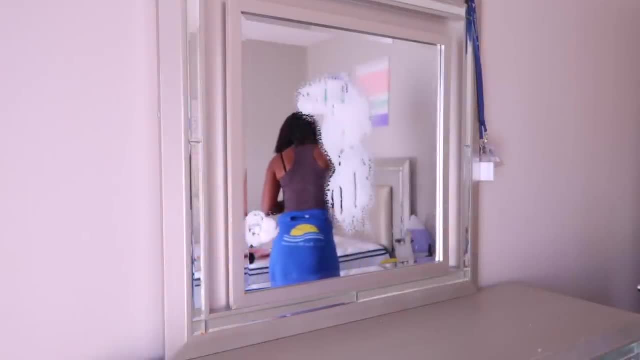 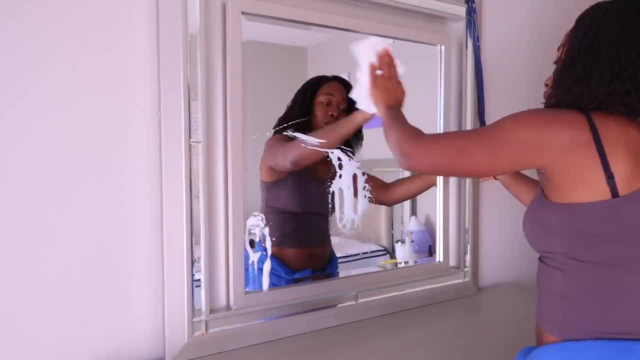 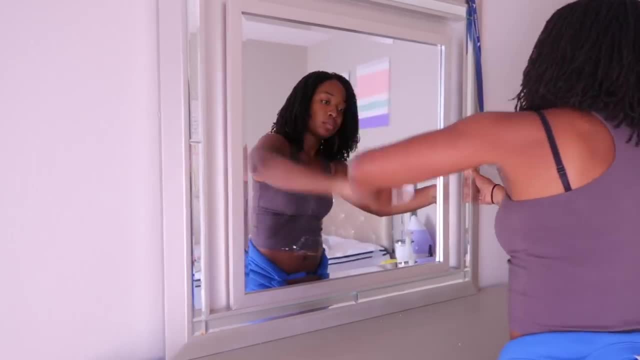 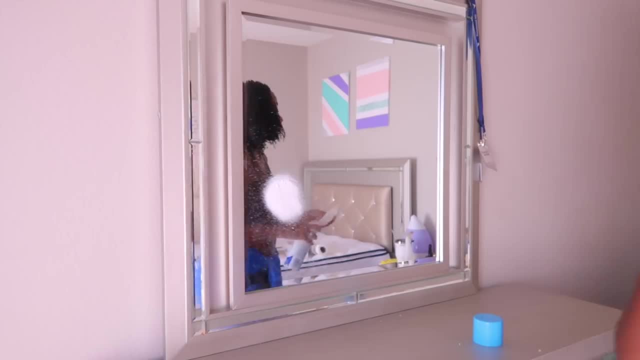 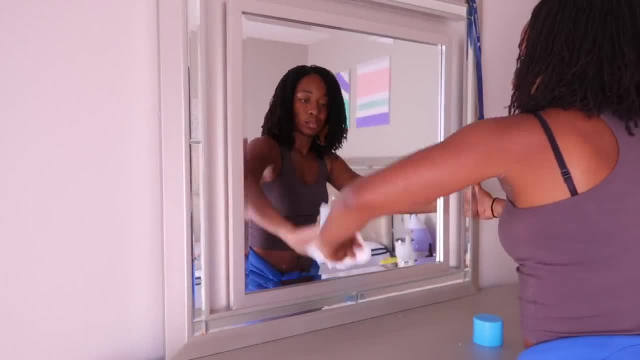 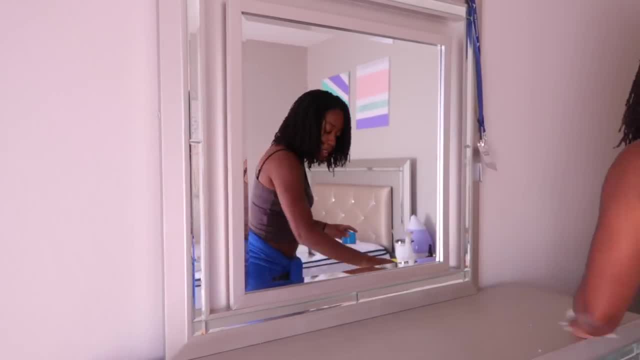 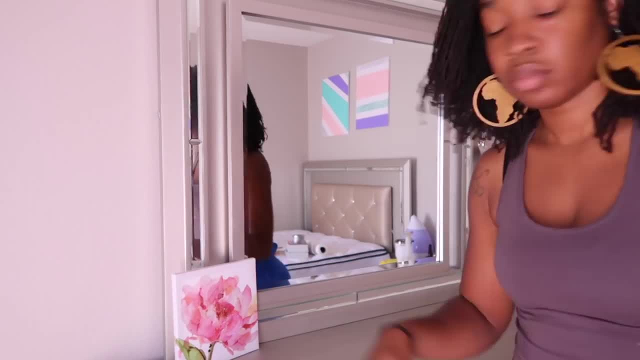 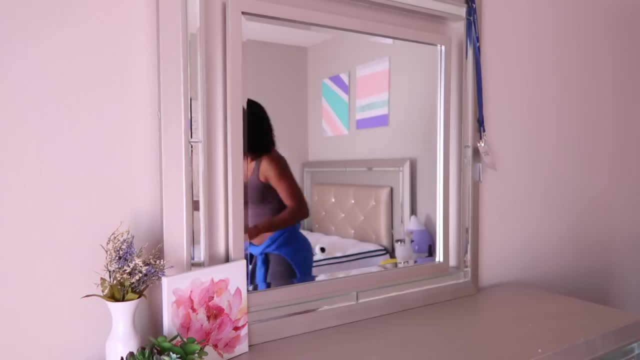 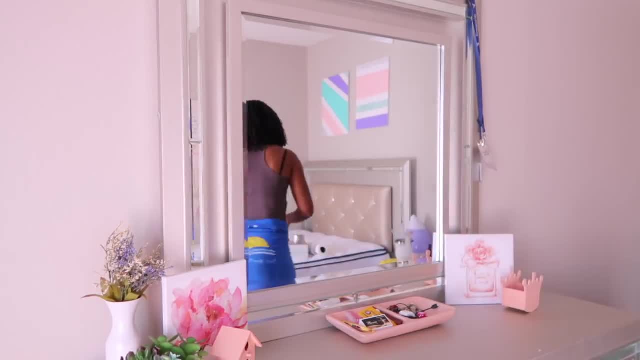 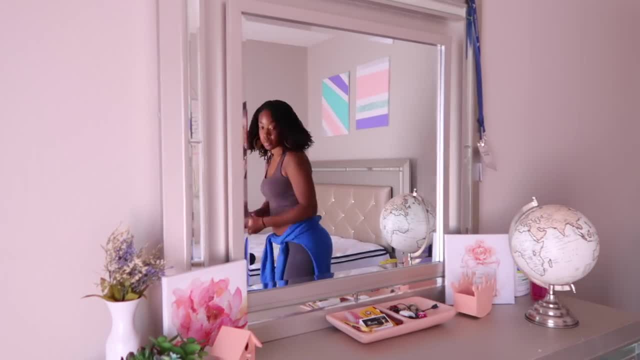 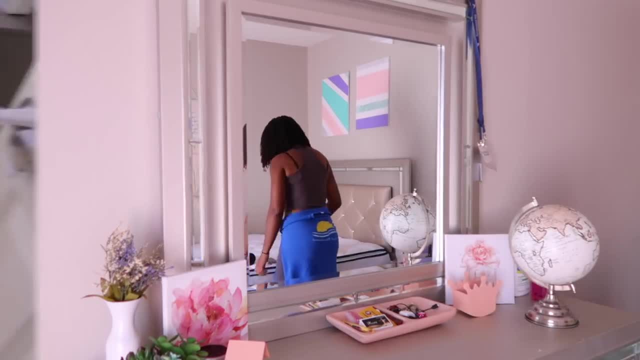 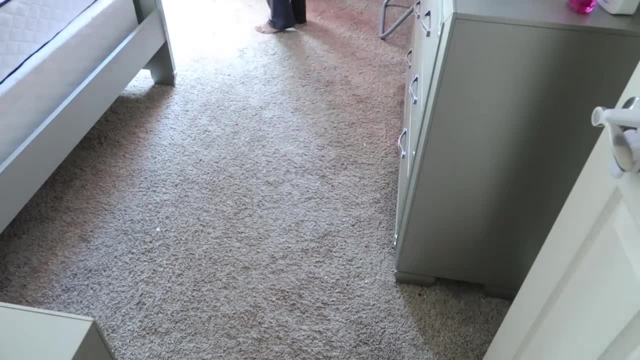 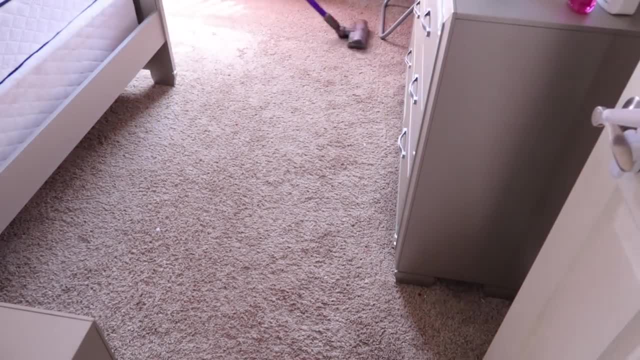 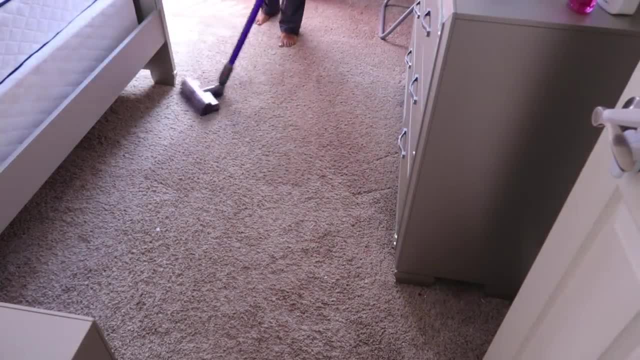 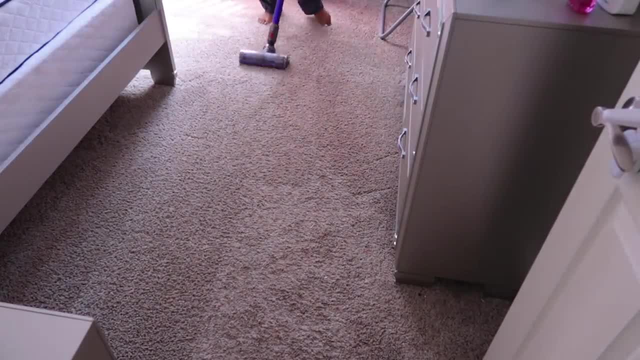 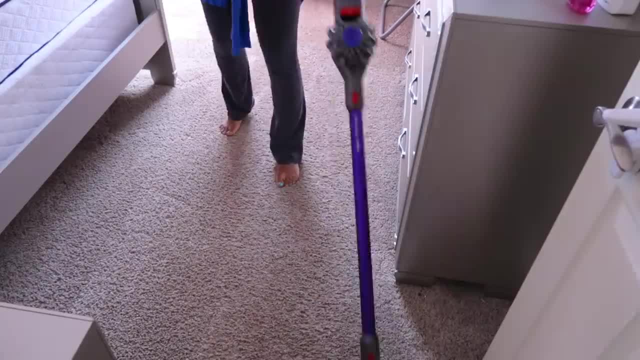 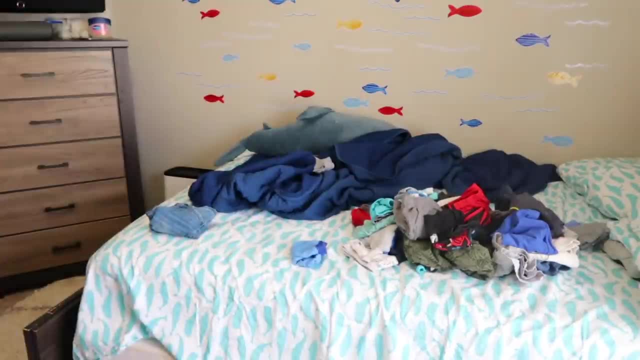 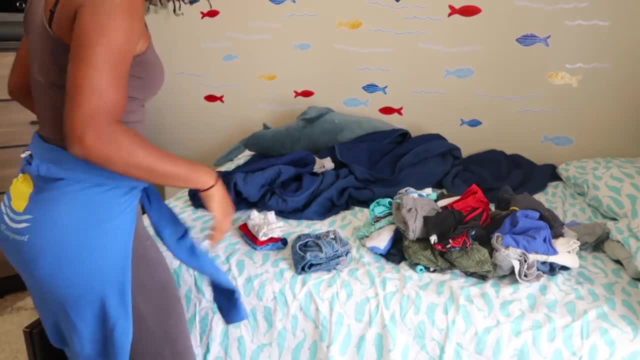 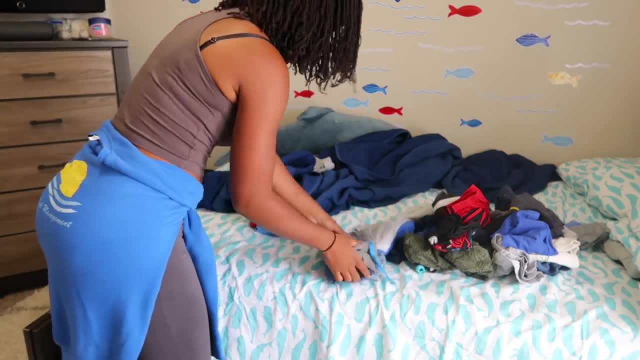 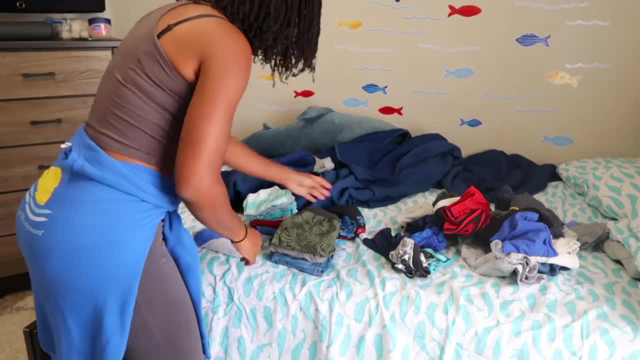 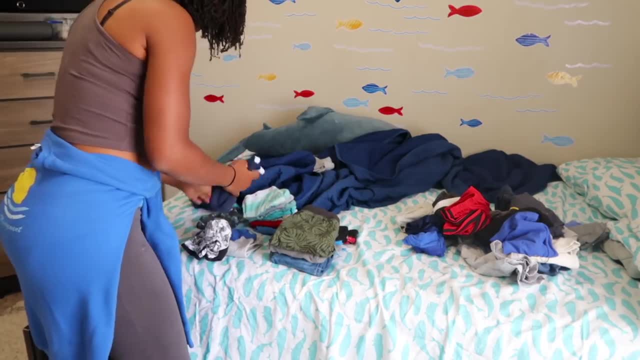 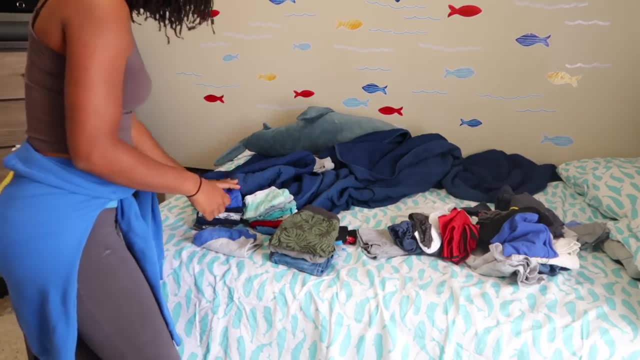 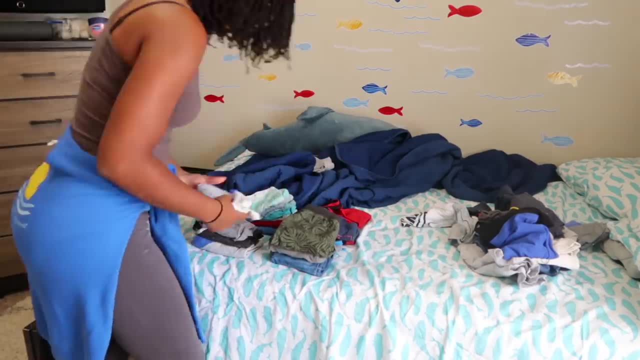 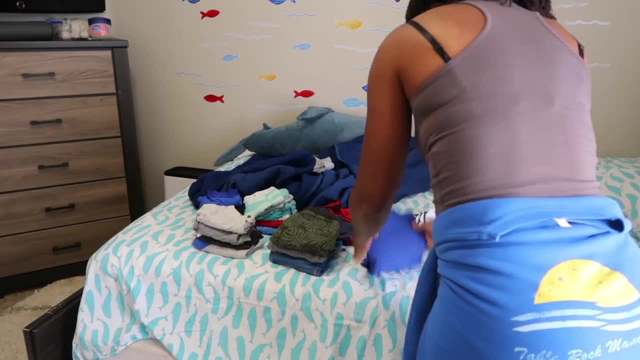 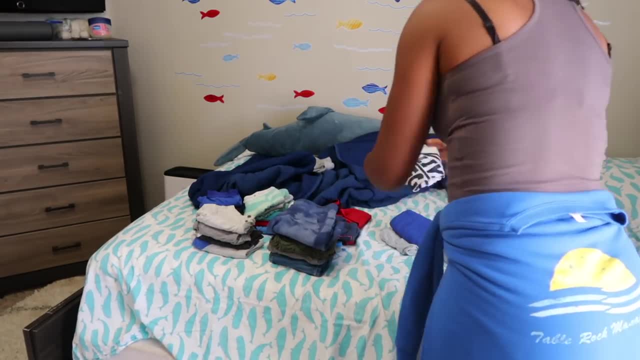 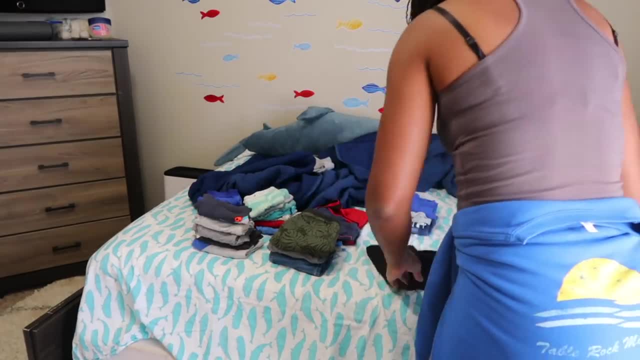 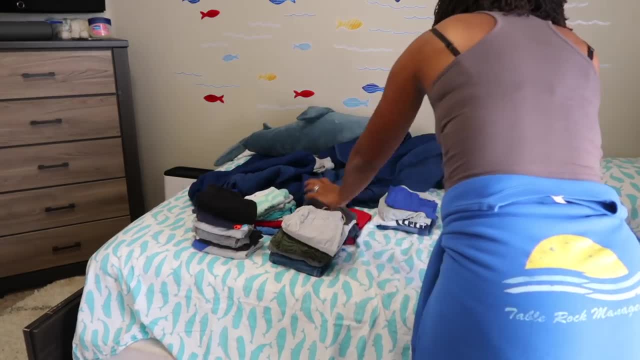 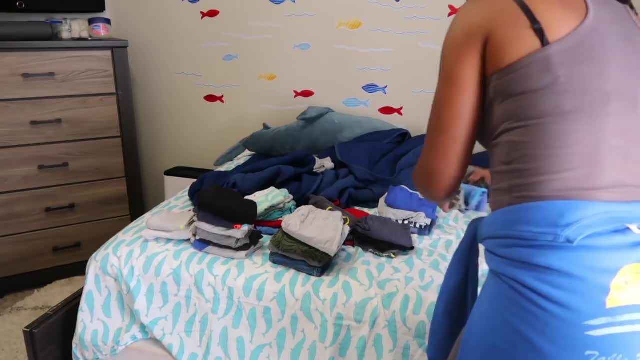 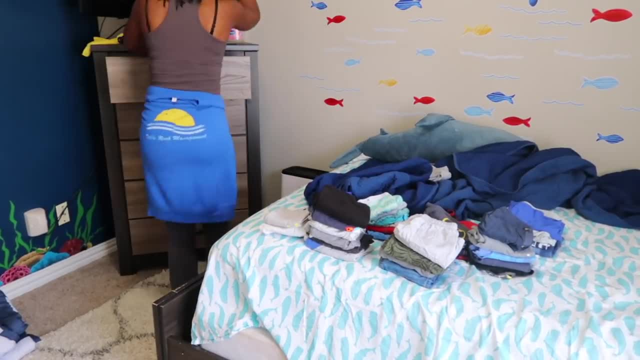 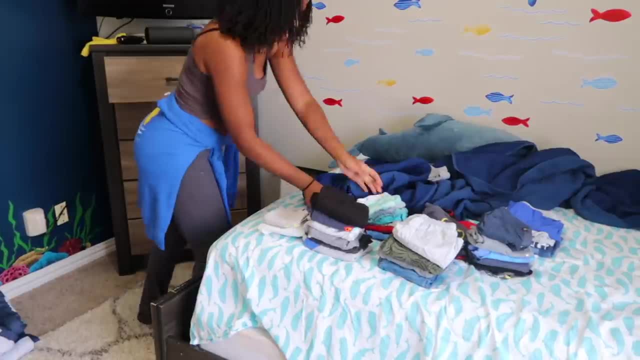 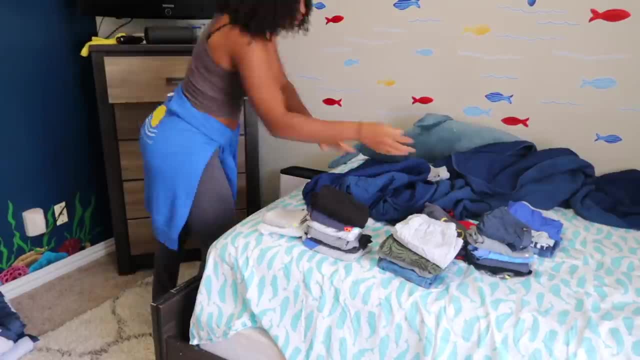 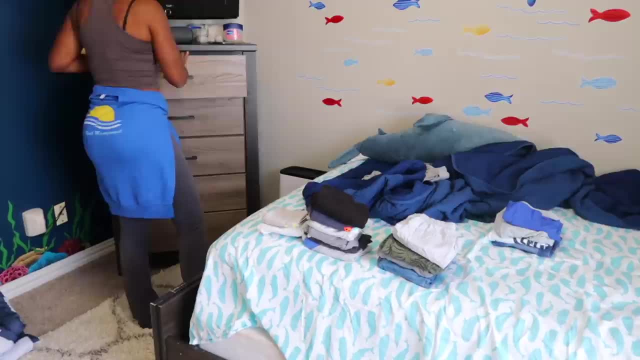 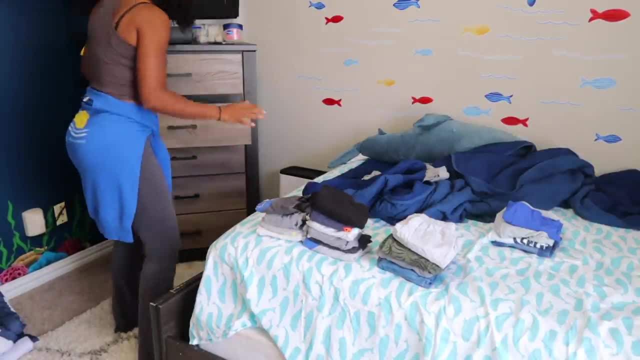 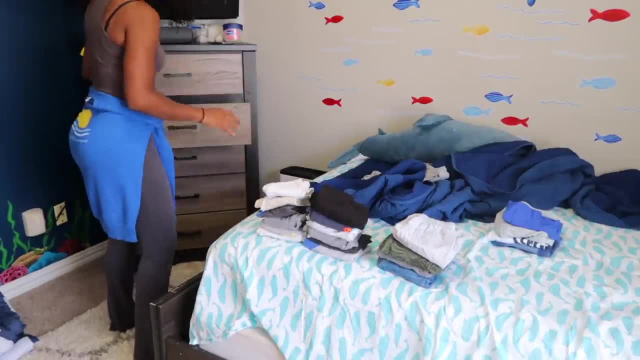 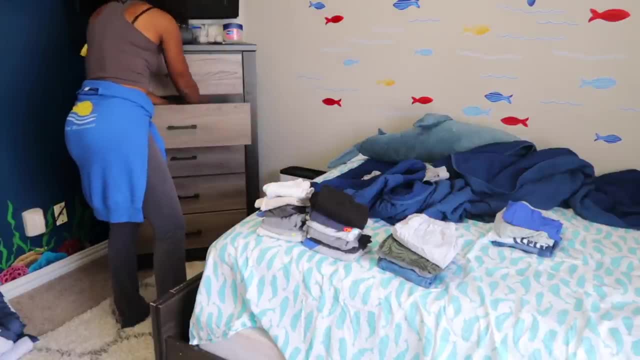 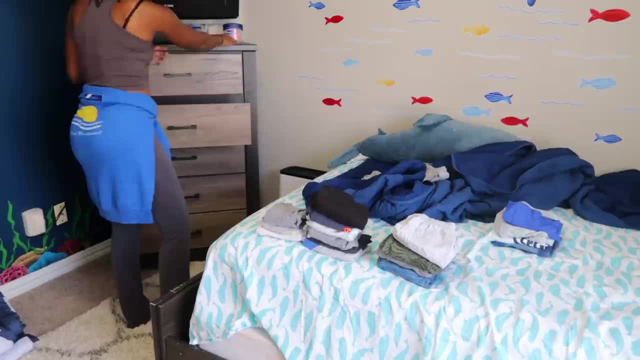 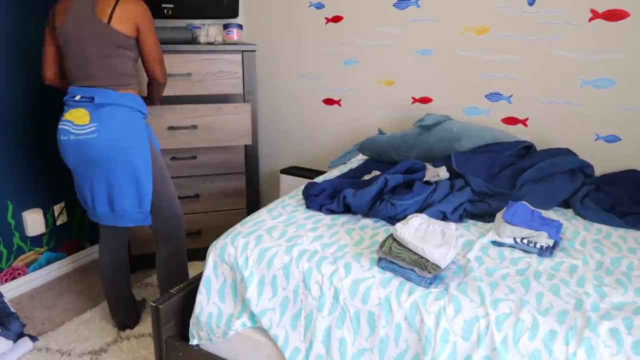 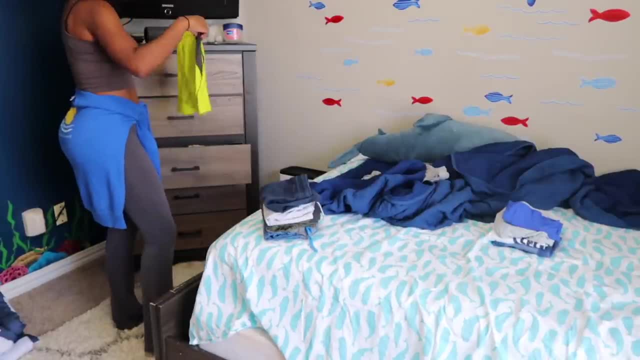 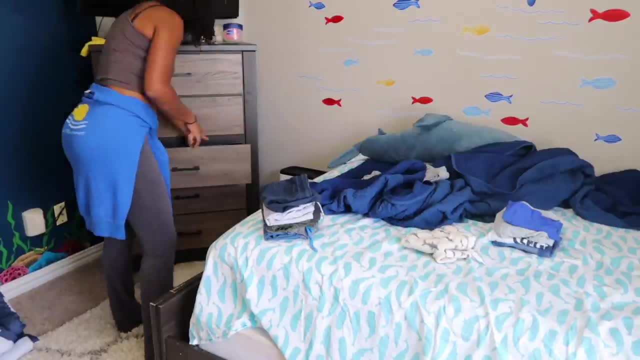 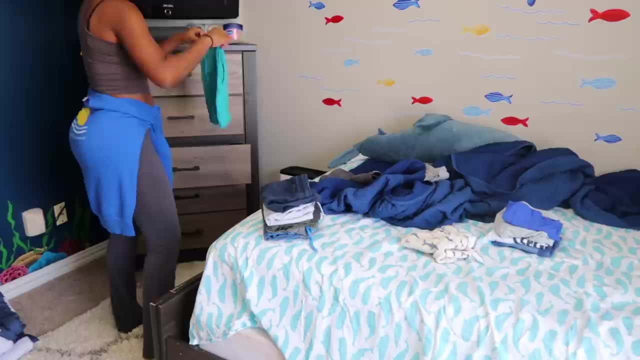 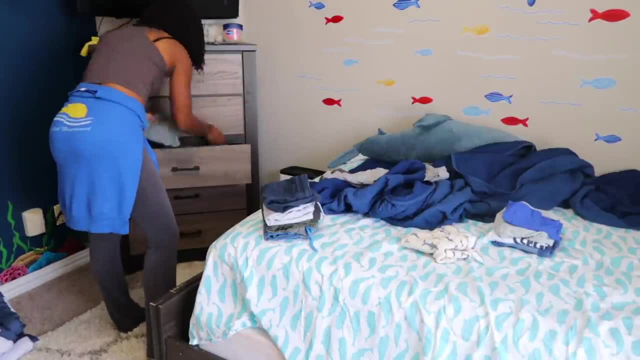 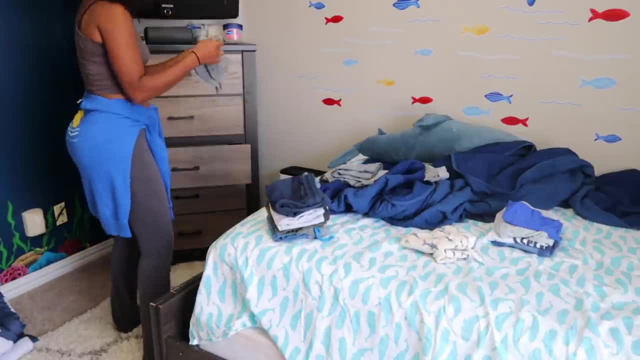 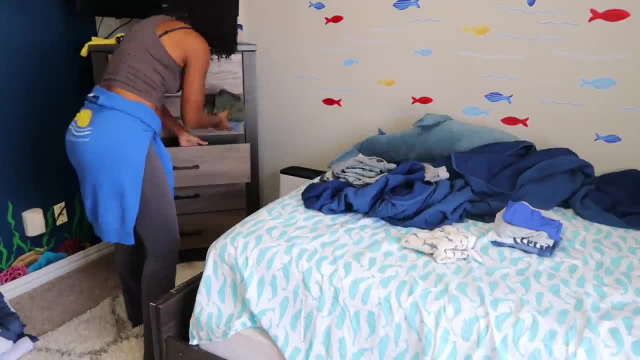 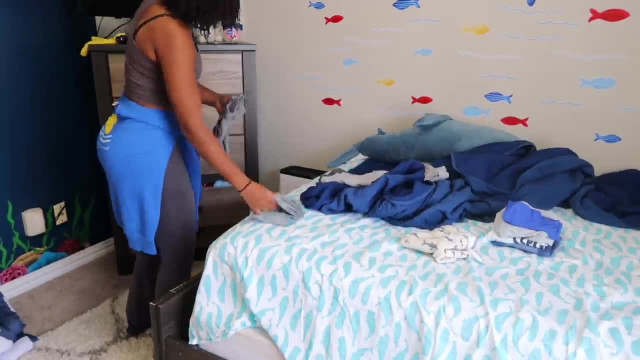 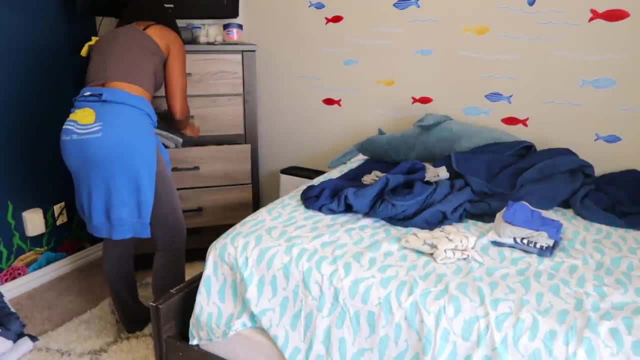 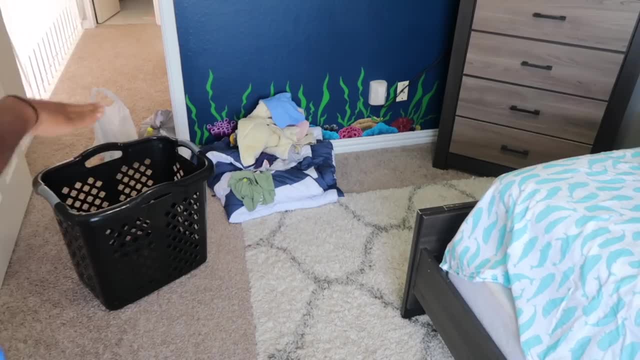 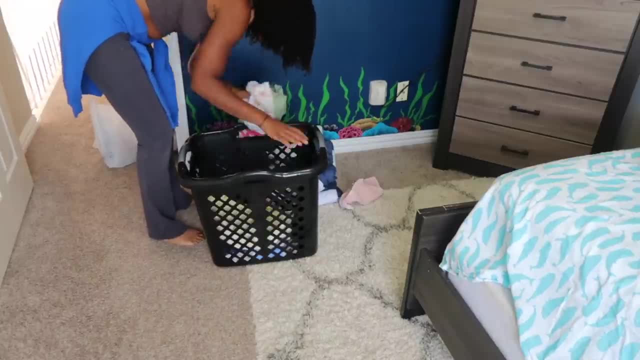 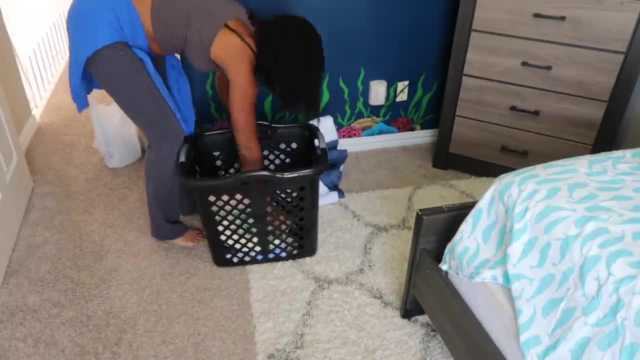 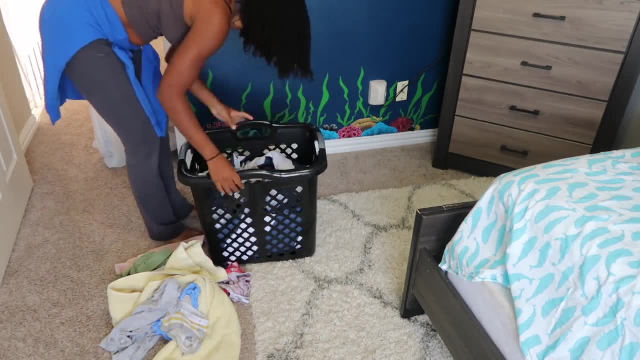 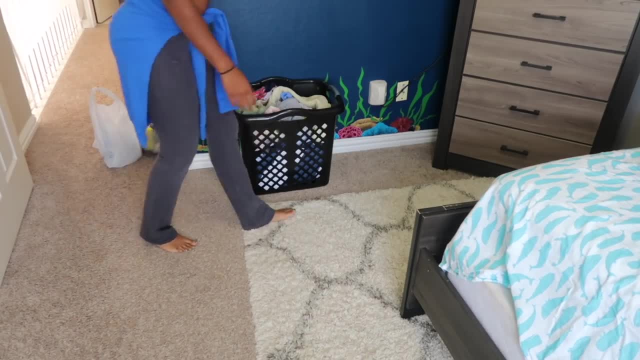 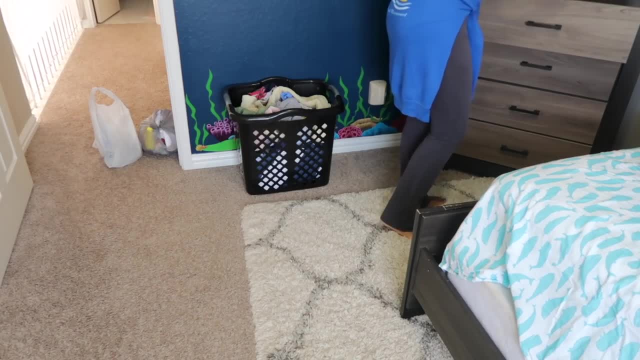 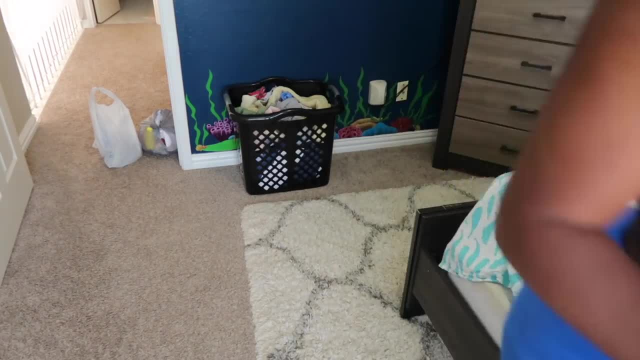 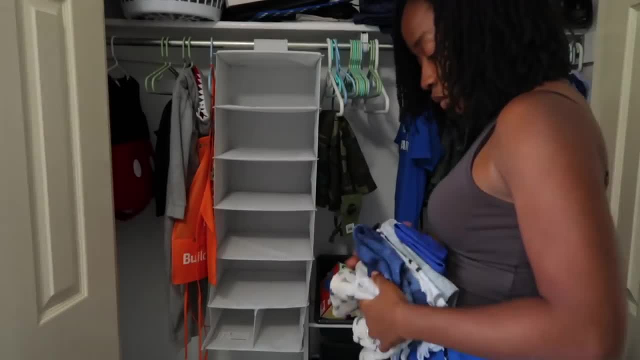 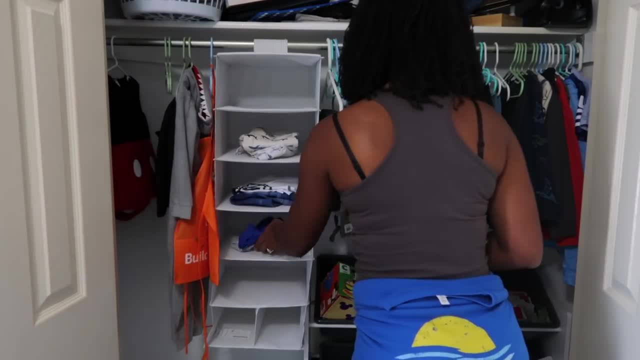 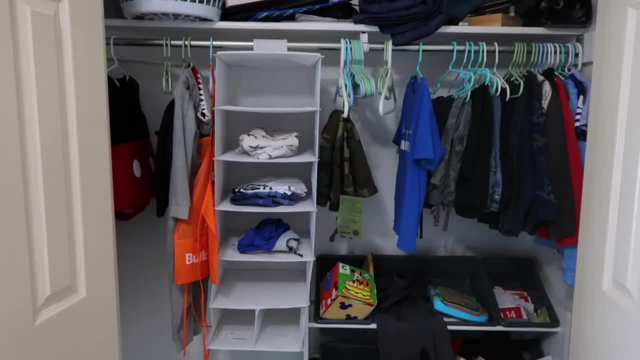 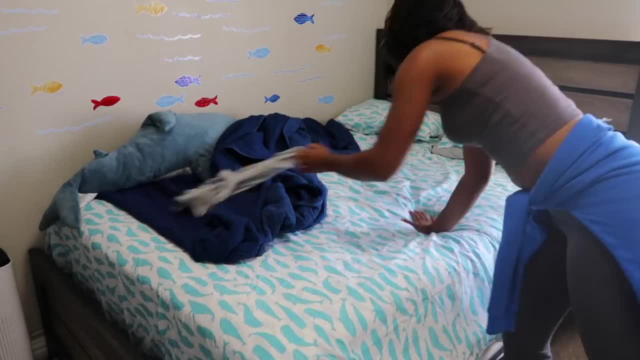 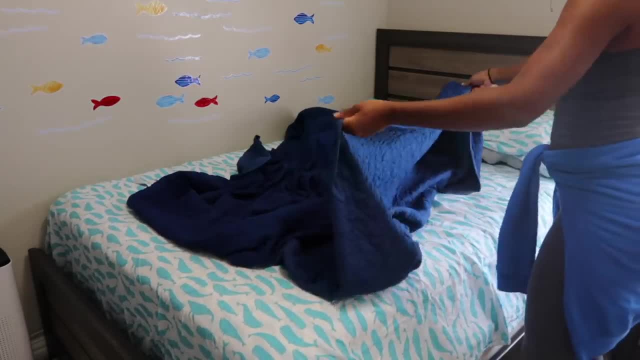 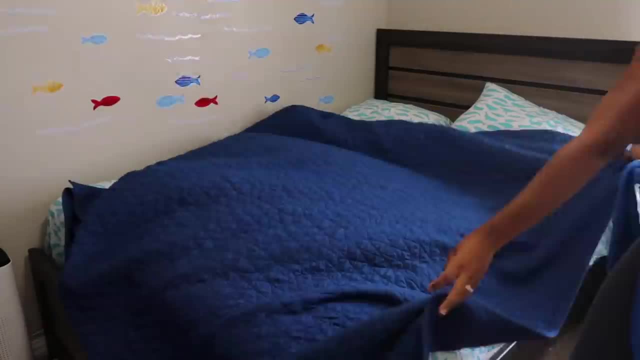 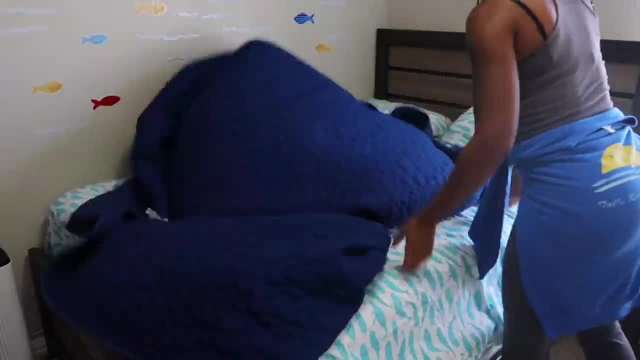 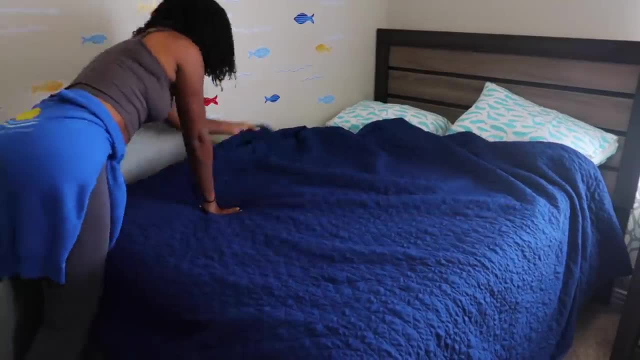 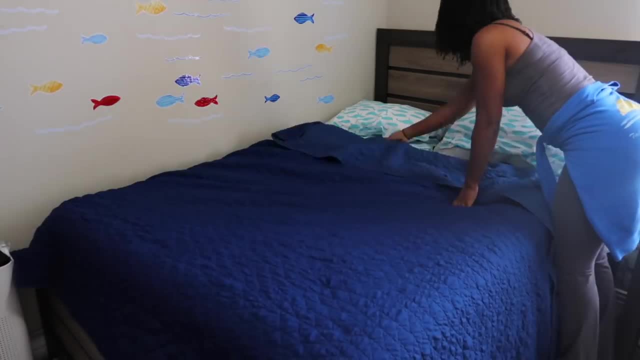 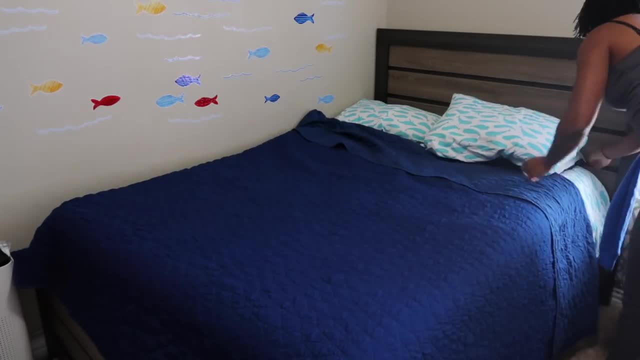 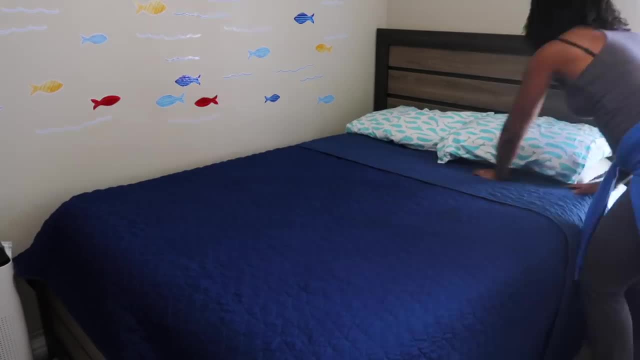 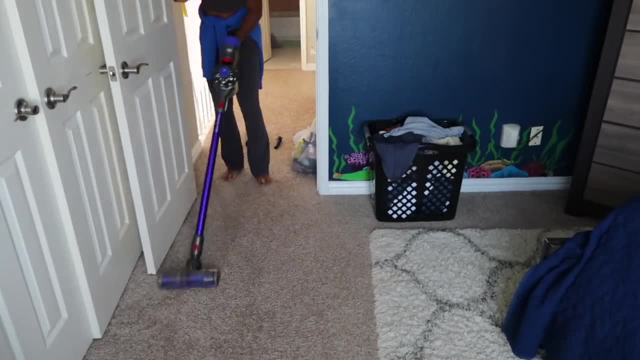 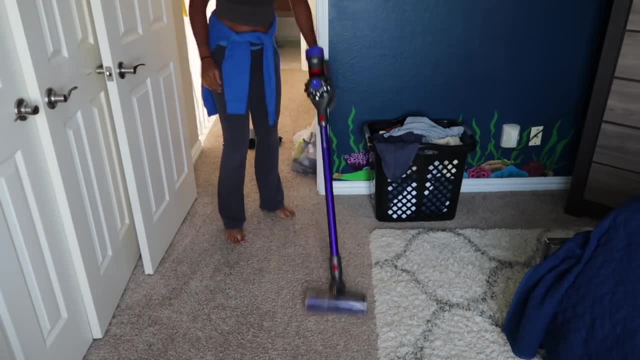 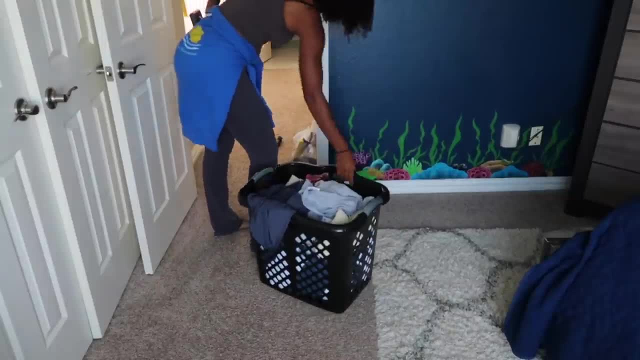 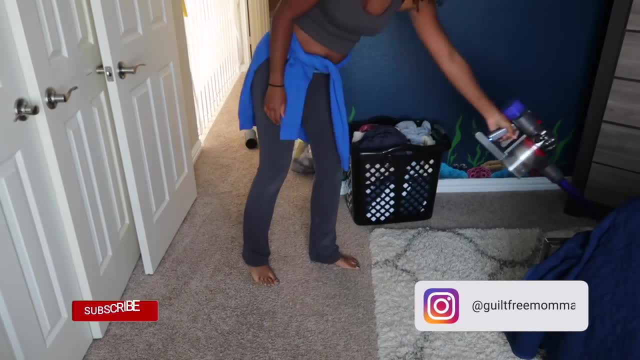 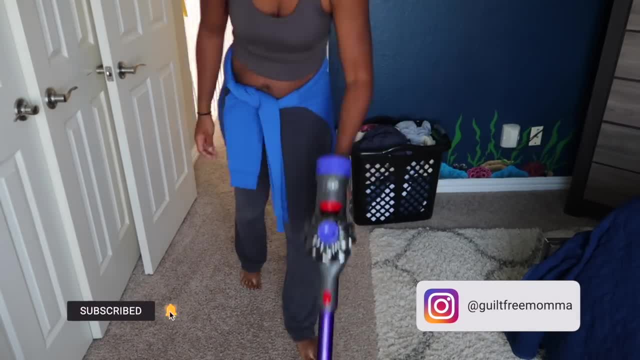 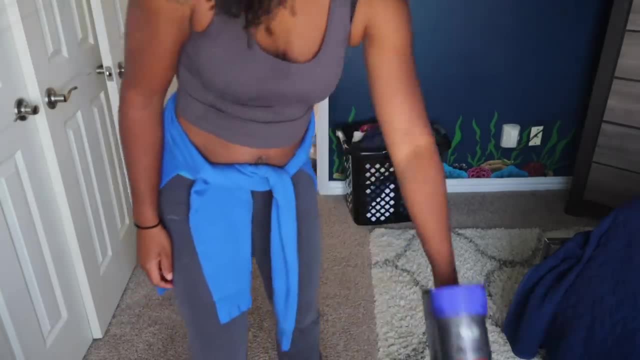 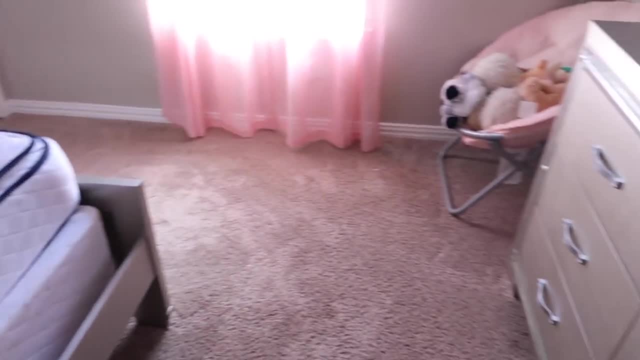 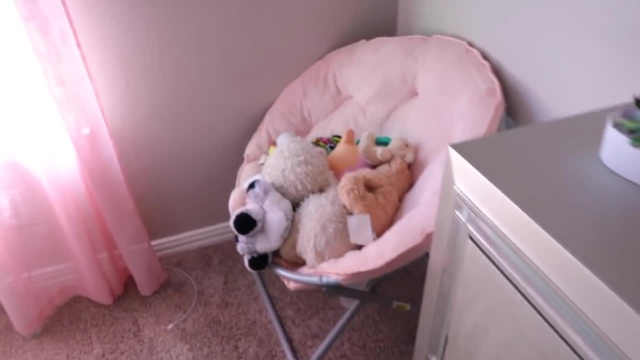 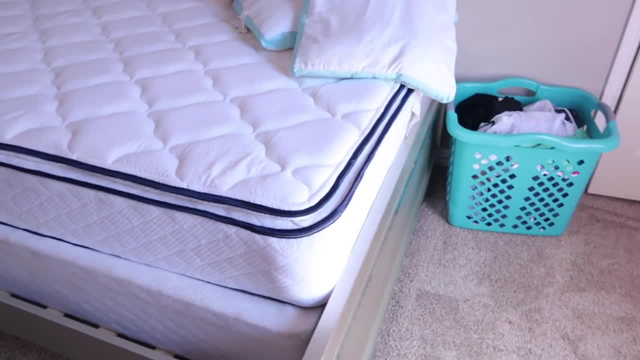 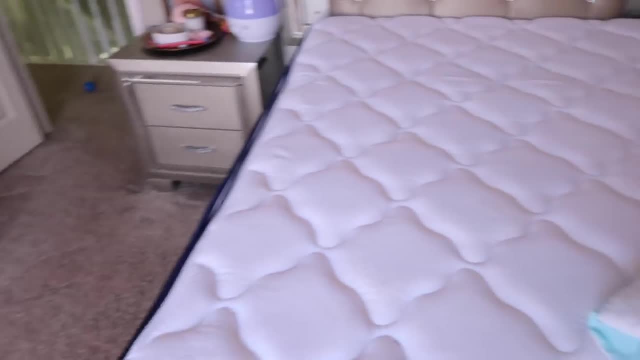 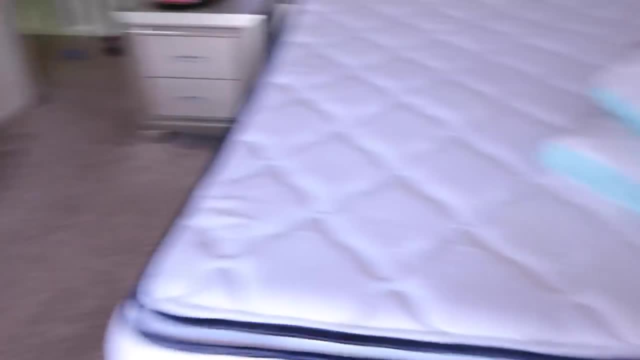 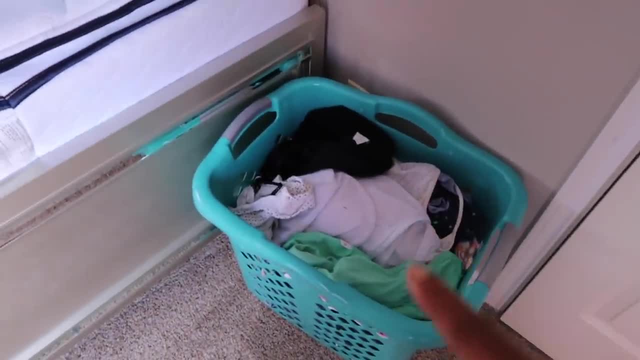 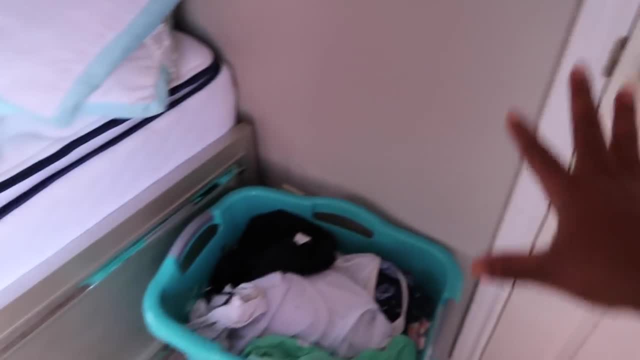 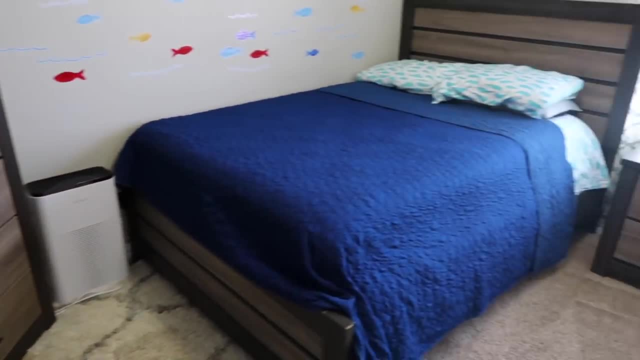 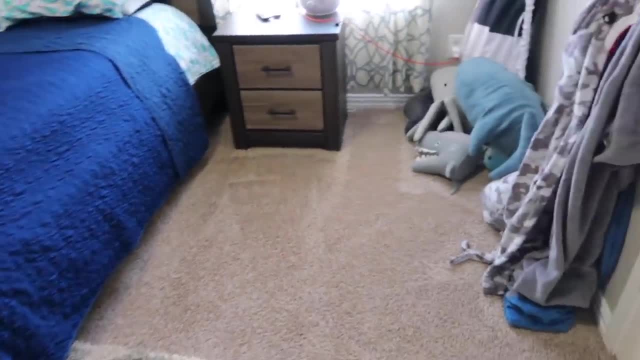